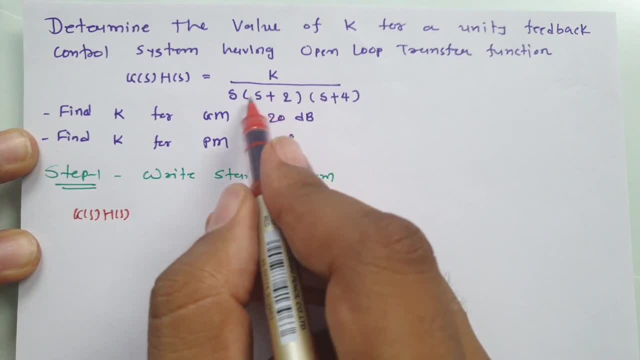 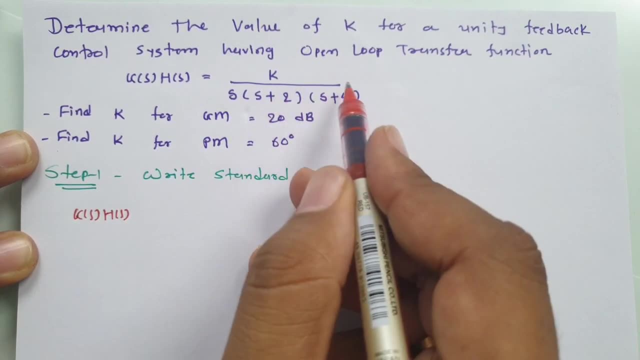 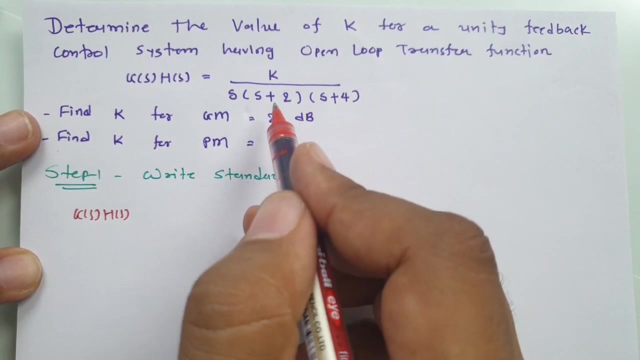 we just need to write this corner frequencies in form of 1 plus s divided by something. so here you see, in numerator there is nothing in terms of corner frequency, but in denominator, s plus 2 and s plus 4 is there. so we need to take 2 and 4 common from this and we can have standard form. 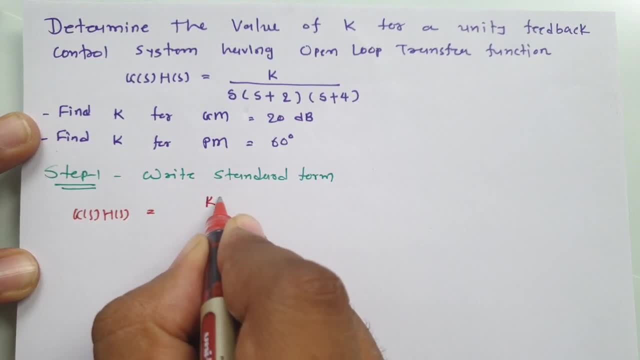 so you see how i am writing it. i am taking 2 and 4 common from denominator, so k by 8, divided by s, into 1 plus s by 2, 1 plus s by 4. see, this is how i am writing standard form right. 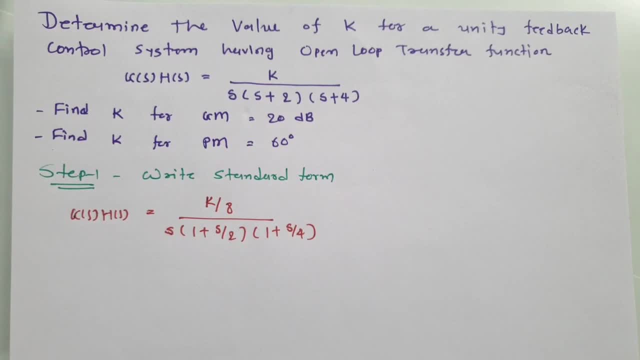 and let us consider here: our constant is k dash, so constant that is k dash, as k is already used. so k dash is equals to k divided by 8. right now, second step is to find slope of first line. so slope of first line that is based on: 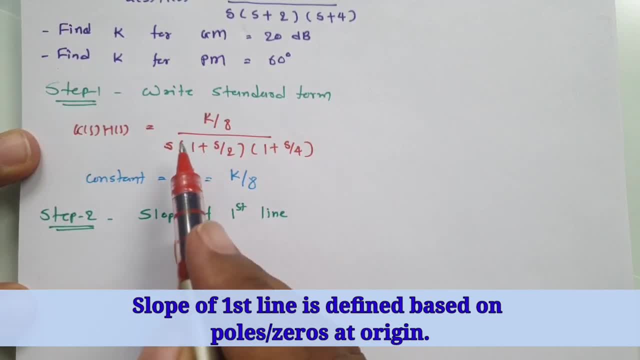 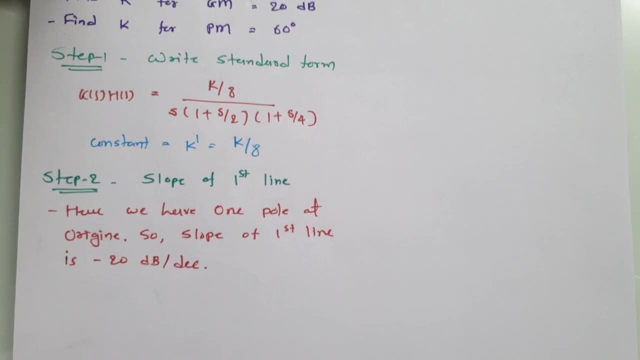 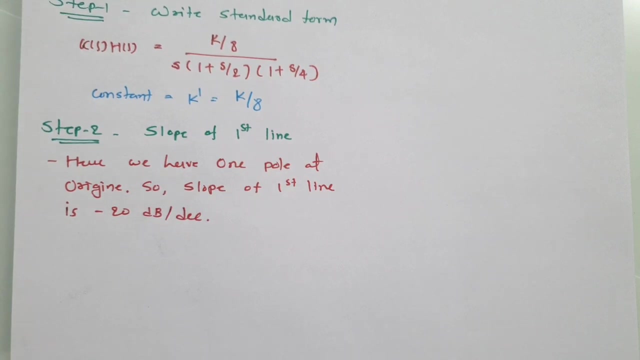 poles or zeros at origin- here you can observe there is one pole at origin- means slope of first line that is minus 20 db per decade right now. third step, that is, to identify gain of first line at omega is equals to 1 radian per second. 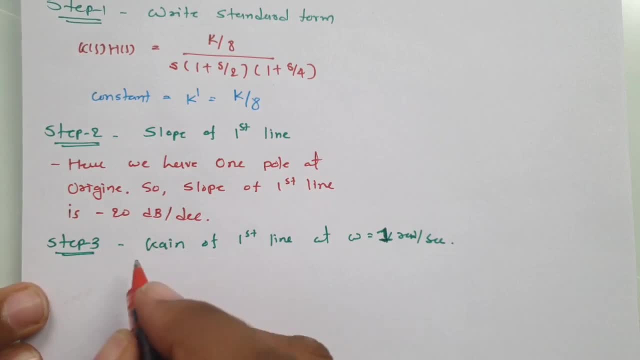 so gain of first line, that is, at omega, is equals to 1 radian per second that we can identify as per 20 log of constant. so here you see, constant is k dash. so i am saying this is k dash and that is 20 log of k by 8, right? 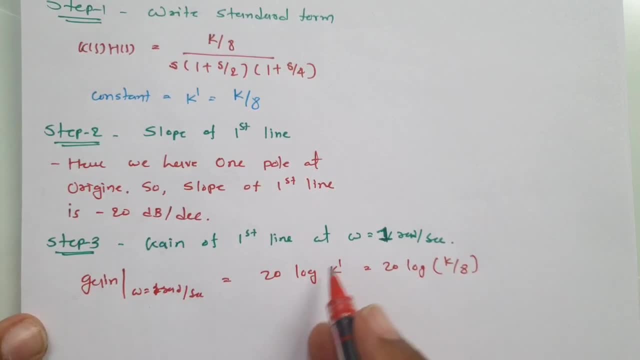 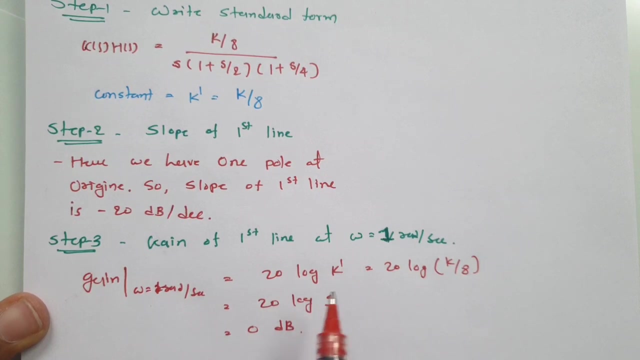 now here: if i consider k dash is equals to 1, right, in that case i can say 20 log of 1, that is 0. so gain of first line: that is 0 db. as we have considered k dash is equals to 1 over here. 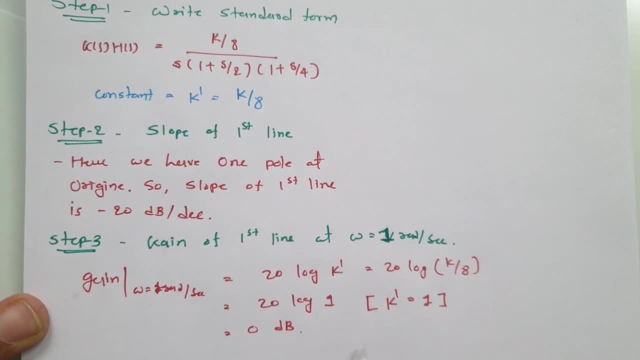 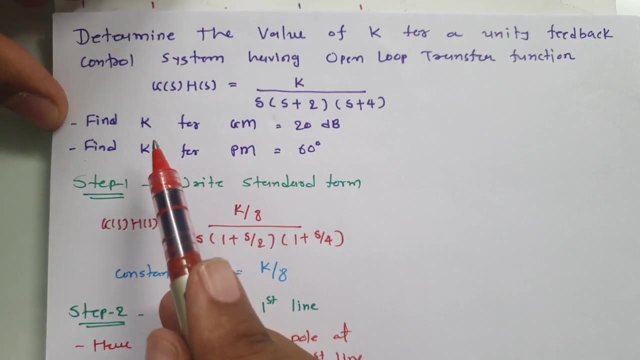 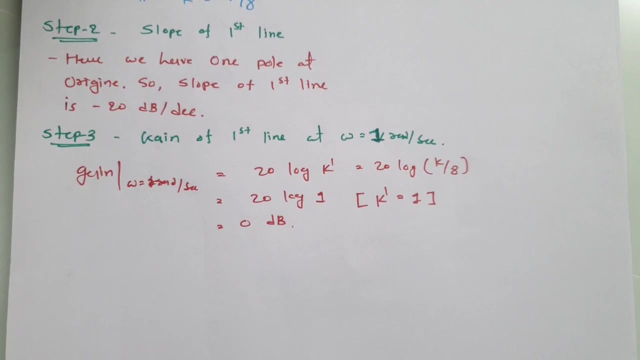 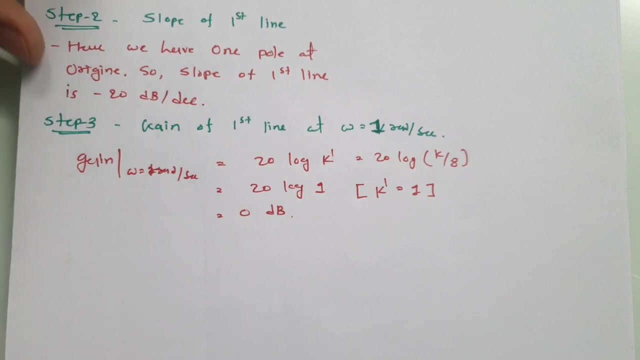 right and by considering k, dash is equals to 1. first we will be plotting body plot, consider this, and after that, based on body plot, we will see how to identify value of k for this gain margin and this phase margin. right now let us see fourth step, and in fourth step we will be writing all 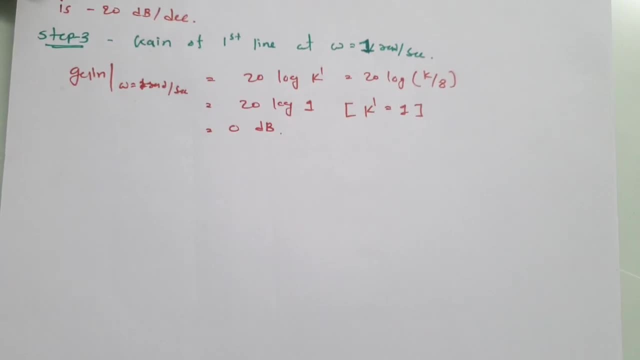 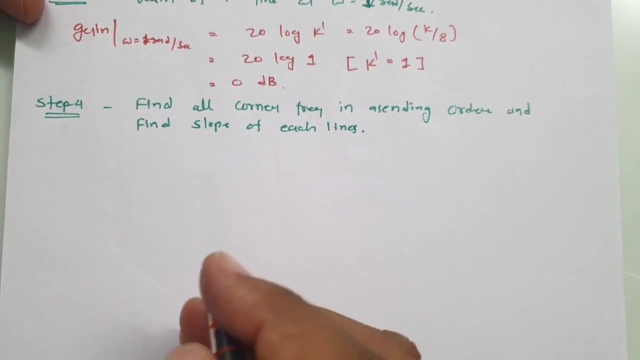 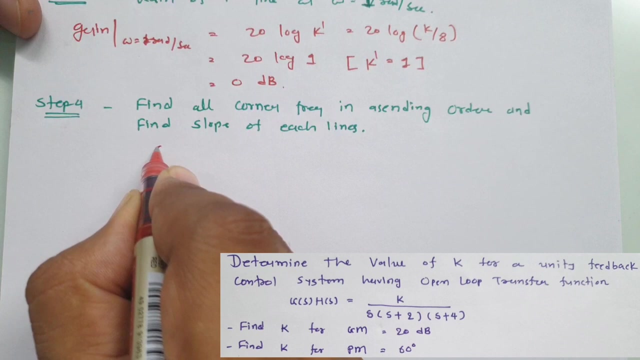 corner frequency in ascending order and we will find a slope of each line. so if you observe our transfer function we will be writing all corner frequency in ascending order and we will find a slope of each line. so if you observe our transfer function then from the transfer function we can say: first corner frequency that is there at origin. 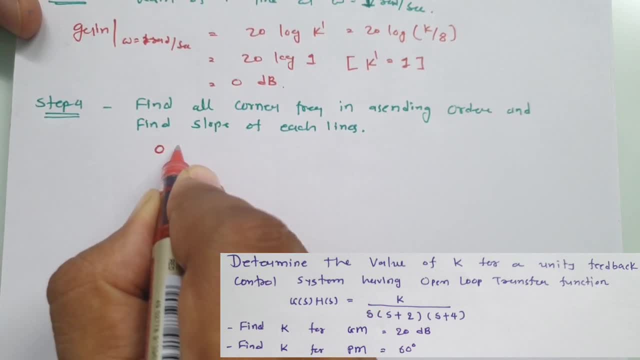 so 0. after that we have second corner frequency that is there at omega is equals to 2, and after that third corner frequency that is happening at omega is equals to 4. so we have three corner frequencies. so i need to write all corner frequencies in ascending order. 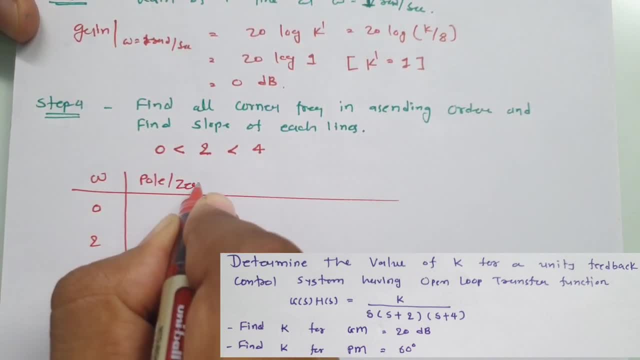 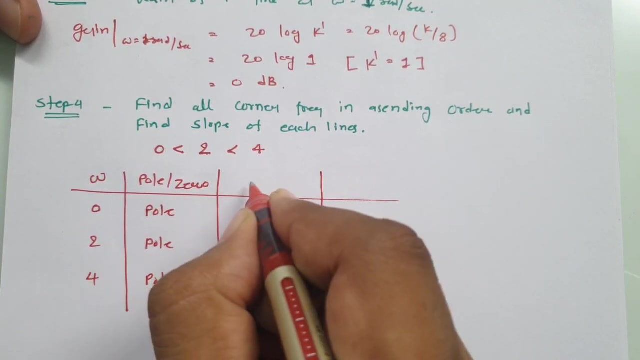 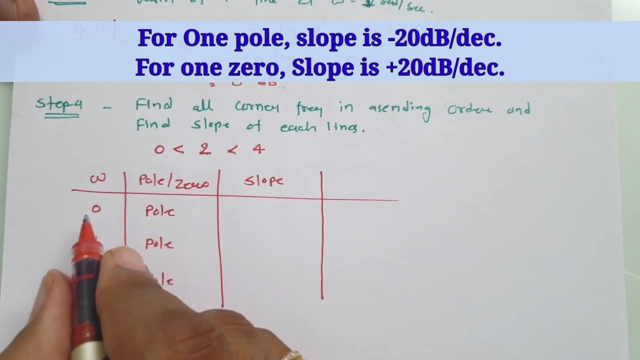 now. next is we need to write pole or zero at each corner frequency, and here, with all corner frequencies, there are poles. so here we need to mention pole with each corner frequency. with pole and zero we have a slope with each line. so if we have one pole over here at origin, we have slope which is minus 20 db per decade. 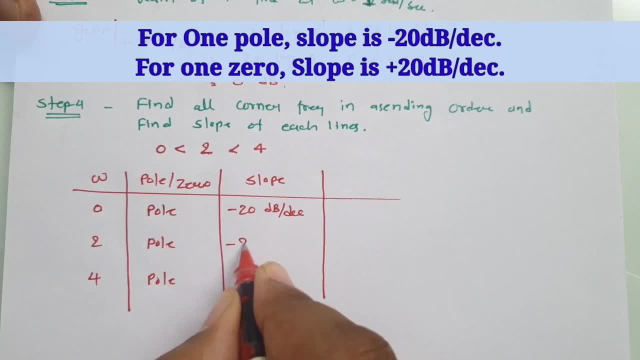 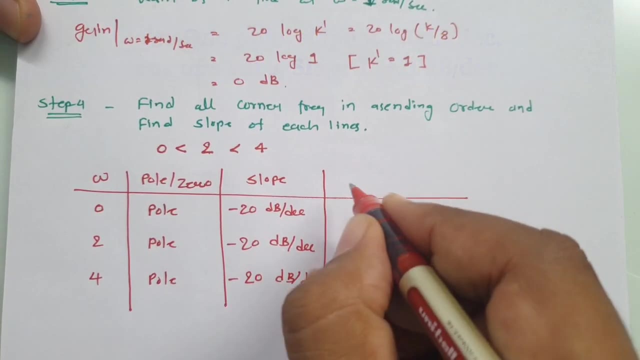 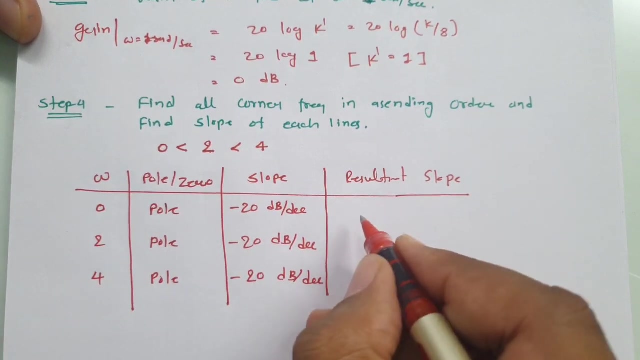 then another pole is there at two, so another slope is minus 20 db per decade. and another slope is, another pole is there at four, so again slope is minus 20 db per decade and here we will be finding resultant slope and first line slope that is minus 20 db per decade. let me keep as it is. 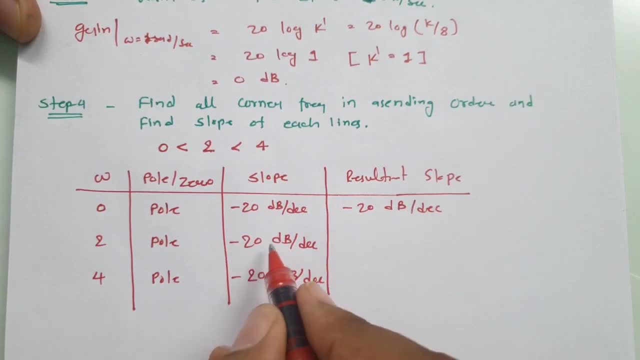 now, next line slope, that is previous one slope plus current slope, so minus 20, minus 20, minus 40 db per decade. next line slope, that is previous slope plus current slope, so previous, is minus 40, minus 20, minus 60 db per decade. see, this is how we can identify slope of each line. so first line slope: 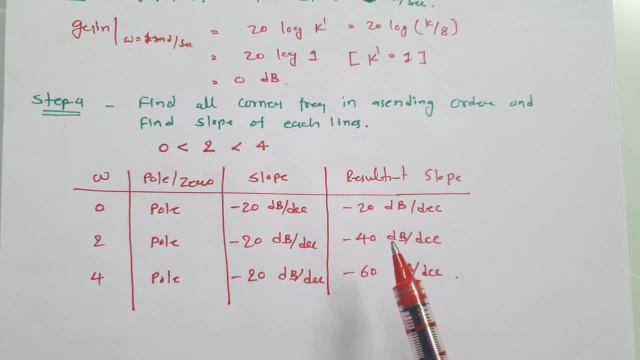 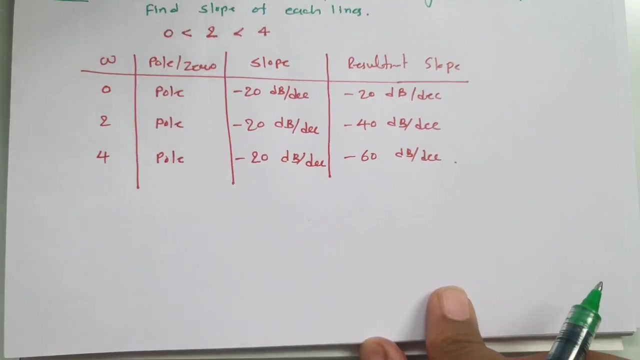 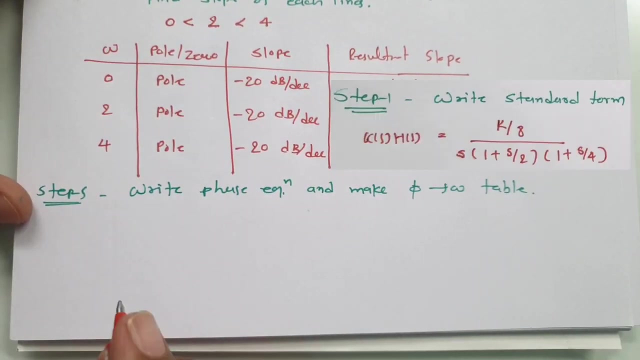 is minus 20 db per decade. second line slope is minus 40 db per decade and third line slope that is minus 60 db per decade. now fourth step, that is, to write phase equation and make a table of phase with respect to frequency. so if you observe our standard form, in that if you place, s is equals. 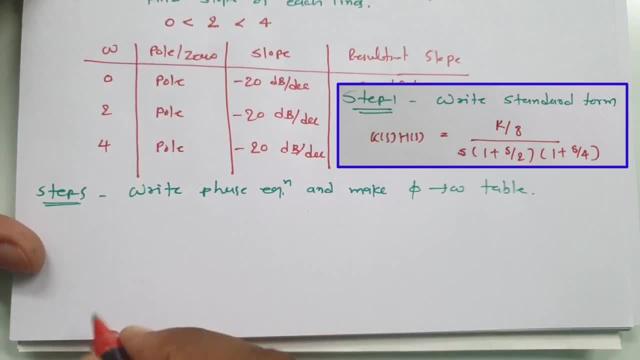 to j omega, then we can have a phase equation and in that, if you observe, at origin there is one pole. so for that slope is sorry, phase is minus 90 degree. and then you see, 1 plus s by 2 means 1 plus j omega by 2 is there and there we have a pole. so 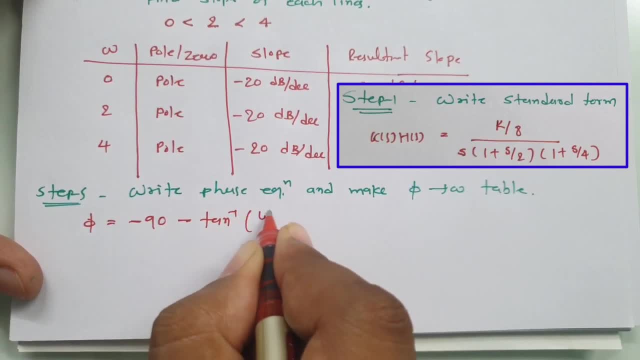 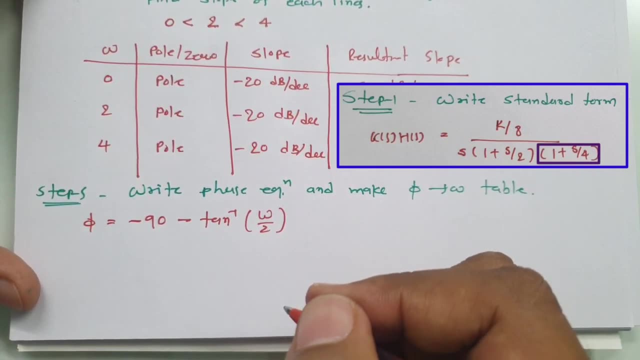 minus tan inverse omega by 2. that is a phase and another corner frequency that is 1 plus j omega by 2. and then we have a phase and another corner frequency that is 1 plus j omega by 2. bye 4 means there is a pole. so minus tan inverse omega by 4, that is the phase which we need to. 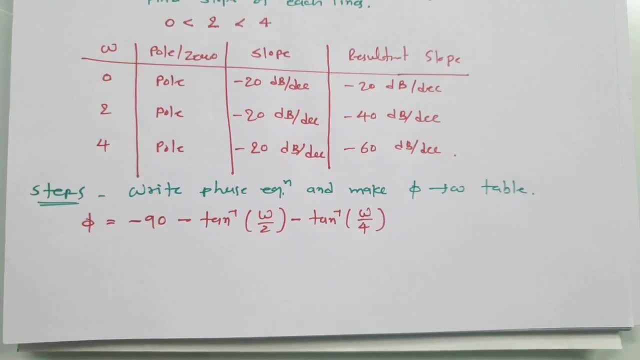 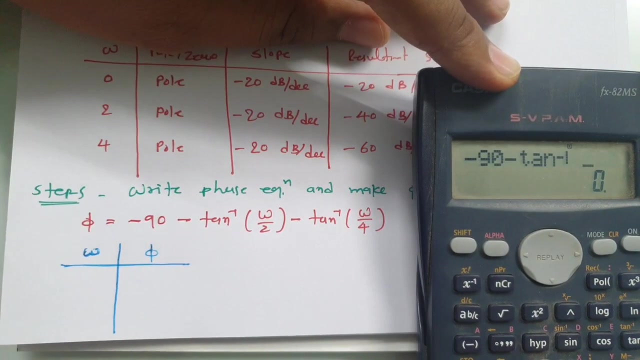 write. now, here we'll be making a table of phase with respect to frequency. so you see, here we have frequency and here we have a phase and we are delivered to have a table of it. so let us Consider first: omega is equals to 0.1 and I am just finding phase. you see, that is minus. 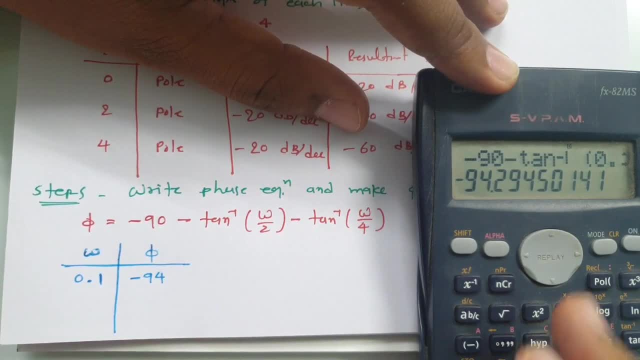 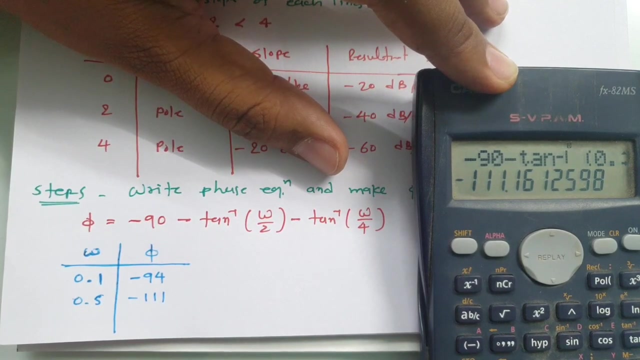 94.. Now, in this same equation, I am just placing: omega is equals to 0.5 and angle is minus 111.. Now next, I am just placing: omega is equals to 1.. So you see 001 that I need to write, and phase is minus 130.. 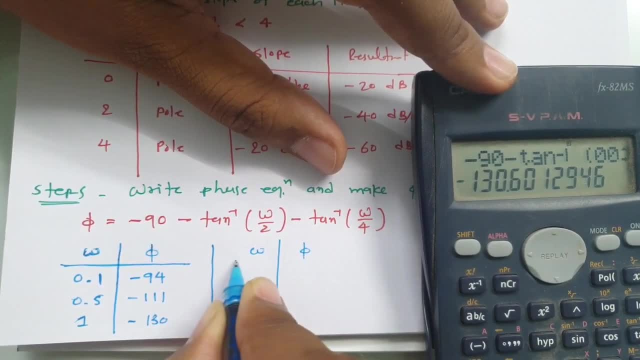 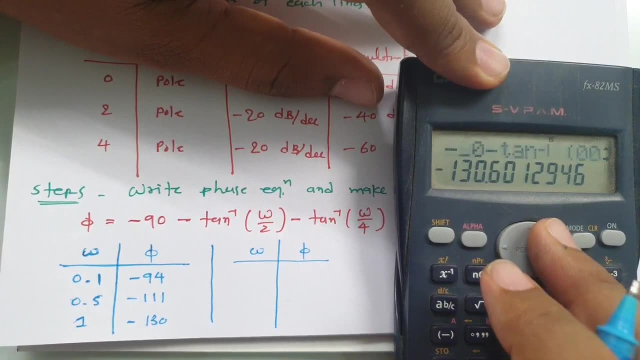 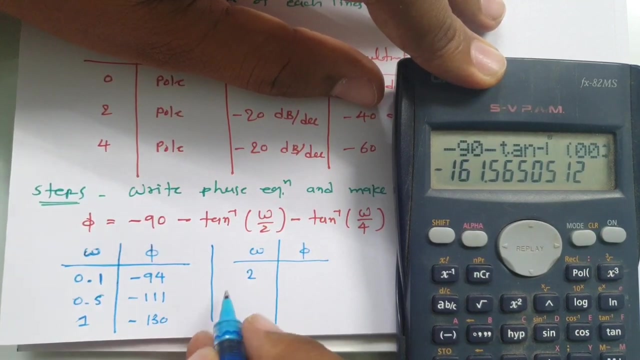 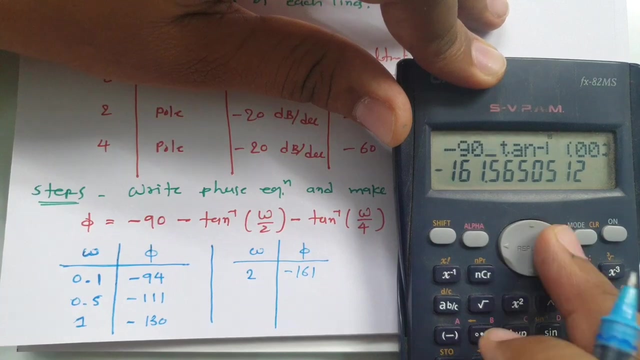 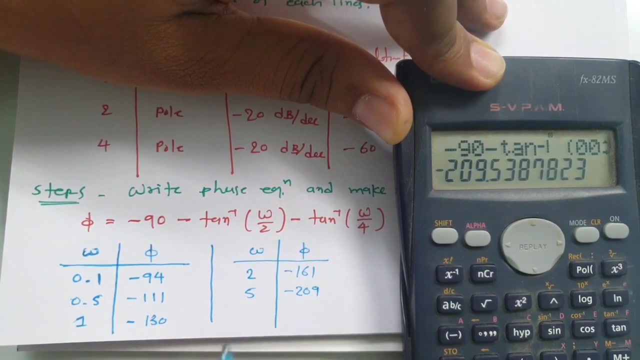 Now few more values that I need to have for omega to have proper plotting of phase with respect to frequency. So let us say We have: omega is equals to 2.. So for omega is equals to 2, phase is minus 161.. Then, for omega is equals to 5, phase is minus 209. 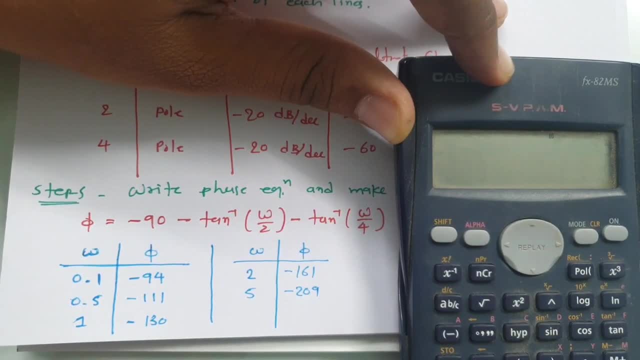 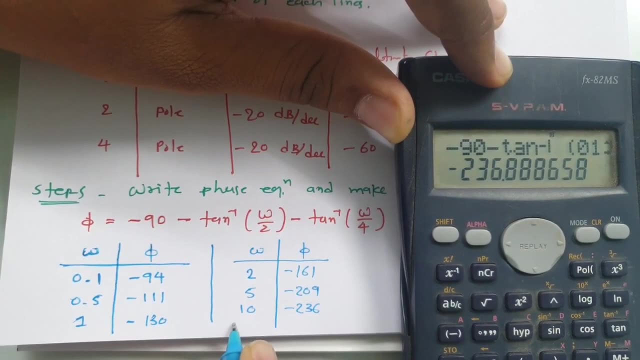 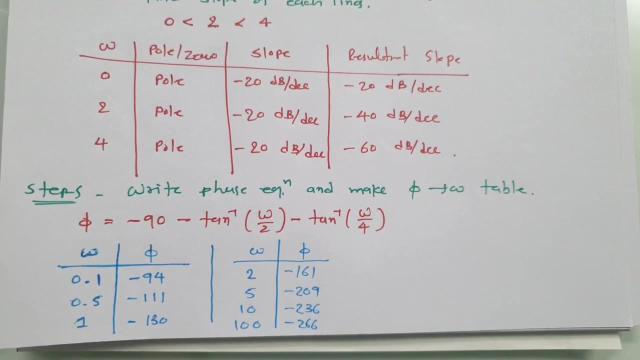 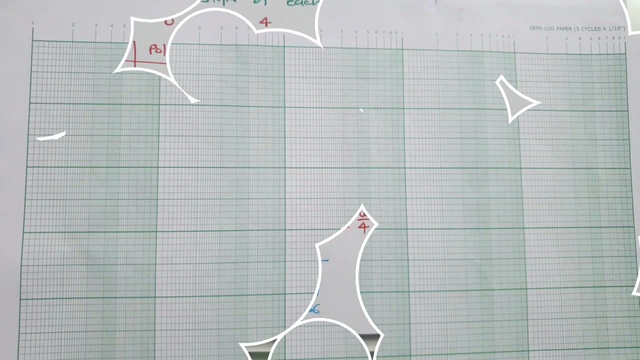 Then omega is equals to 10. Phase is minus 236.. And now I am taking omega is equals to 100.. Phase is minus 266.. So this is how we have a phase table with respect to frequency. Now I will plot for this, given data which we have calculated right now. 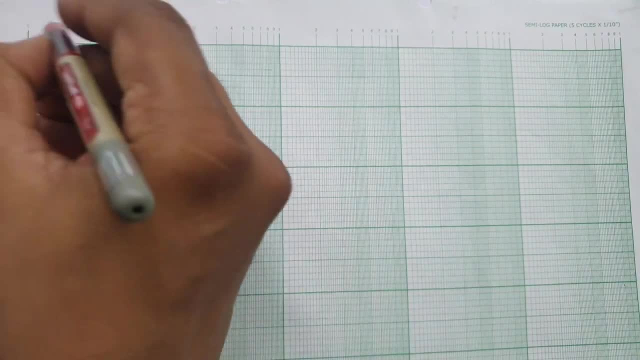 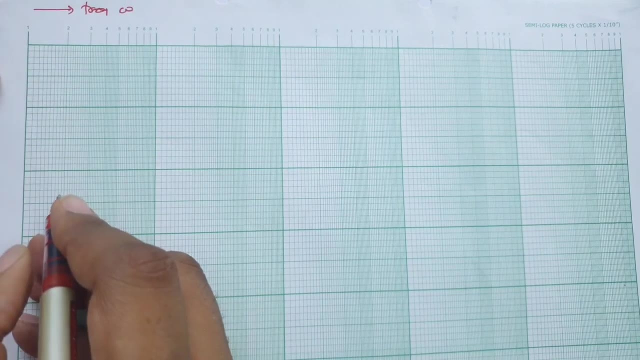 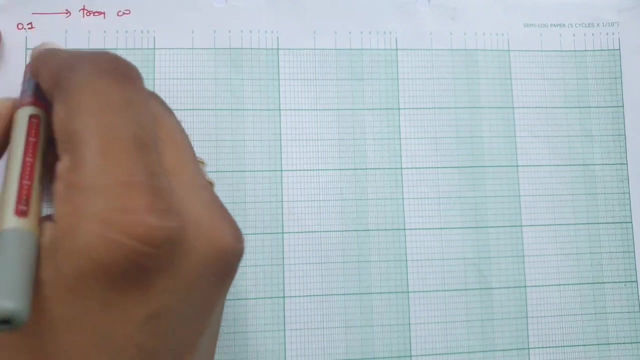 So see, this is semi log graph paper Which we have, and here we have frequency on this axis. Let us say this is omega. Now, here you see: first I am considering frequency 0.1 over here and on this semi log graph paper, you see, this is 1, 2, 3, 4, like this: 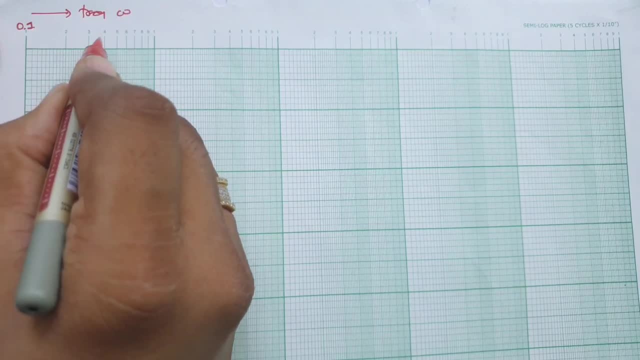 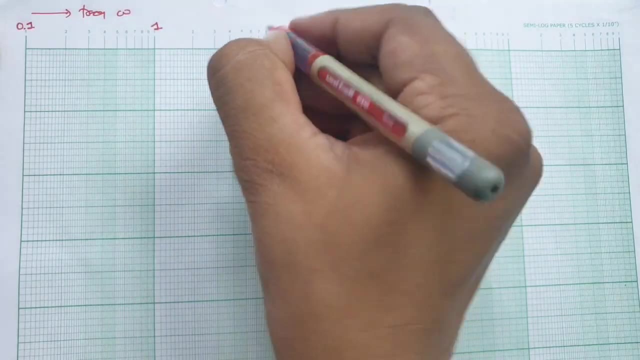 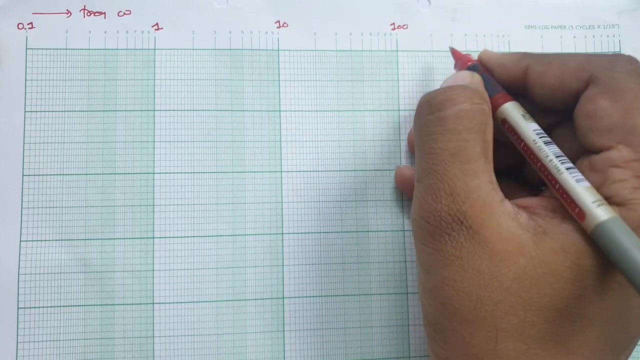 So if this is 0.1, this has to be 0.2, 0.3, 0.4. likewise here it will be 1.. Then 1, 2, 3, 4. likewise here it will be 10.. Then 10, 20, 30, 40. likewise here it will be 100.. 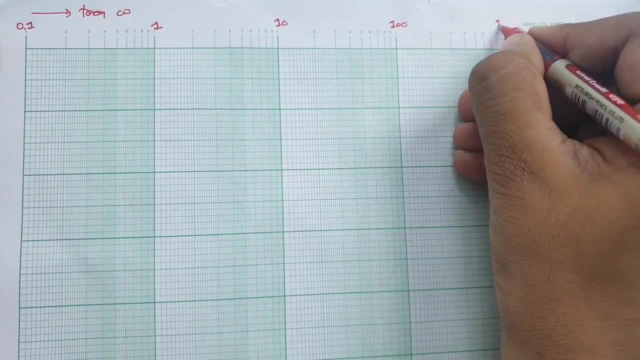 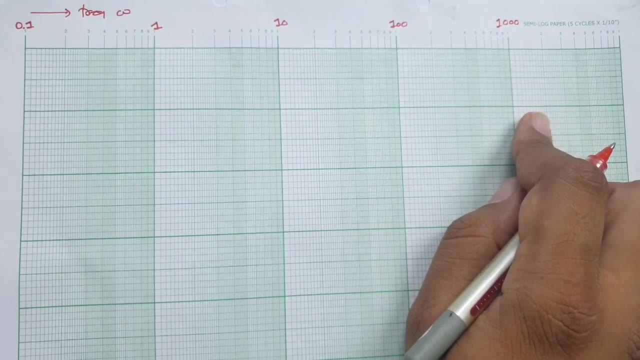 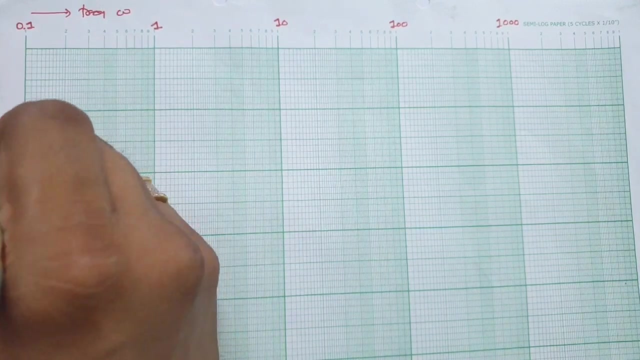 Then 100, 200, 300, 400, likewise it will be 1000.. See, this is how semi log graph paper that we have right, And first we will be having a plot of gain right. So here, all I am considering is, This is our gain plot. 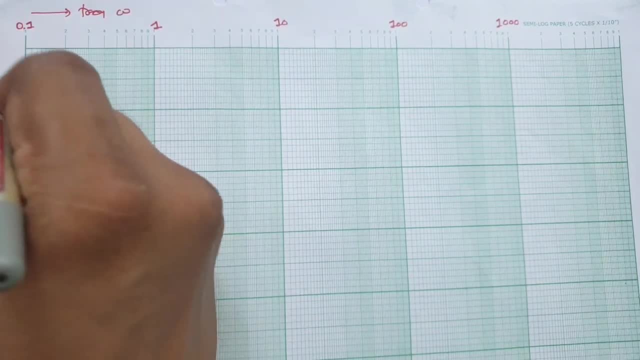 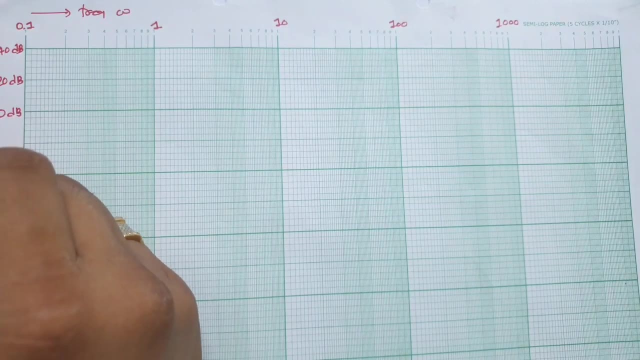 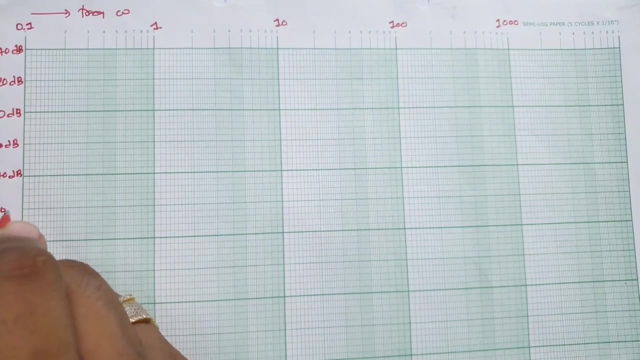 Where 0 dB that I am considering over here, And here there is 20 dB, and here there is 40 dB, And here there is minus 20 dB, minus 40 dB and minus 60 dB. That is how it is there with us, right. 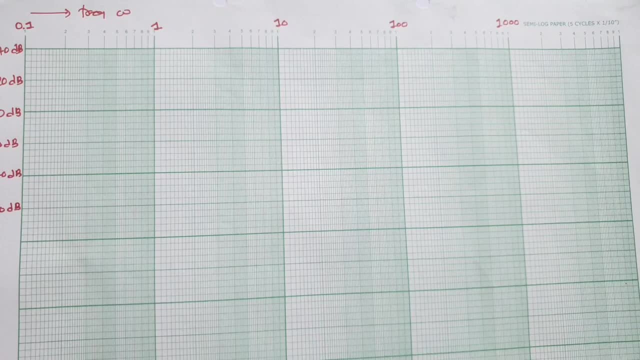 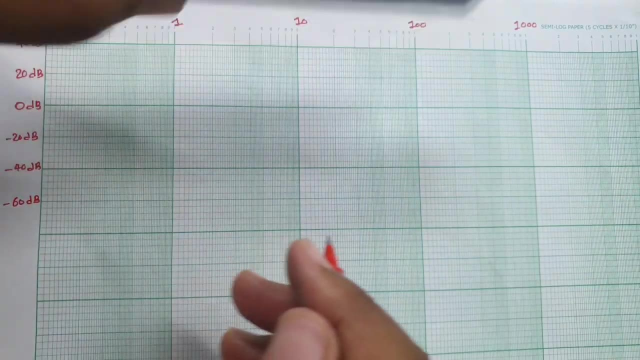 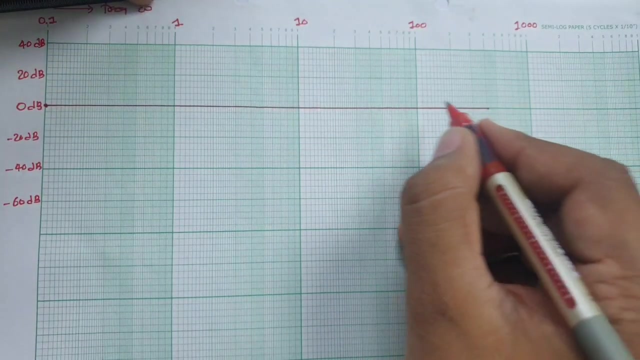 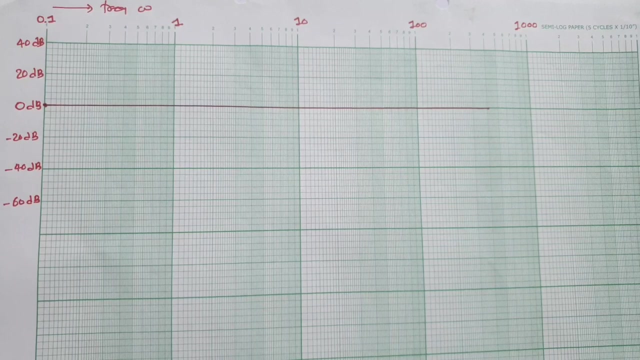 And first we need to have this 0 dB line Extended Right, Right Extended over this side, Right As gain cross over frequency. that is happening at 0 dB. I am just extending 0 dB line like this. Now let us try to understand what will be our first line as per the calculation. 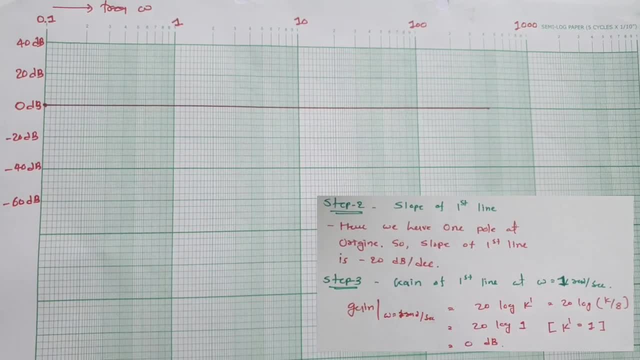 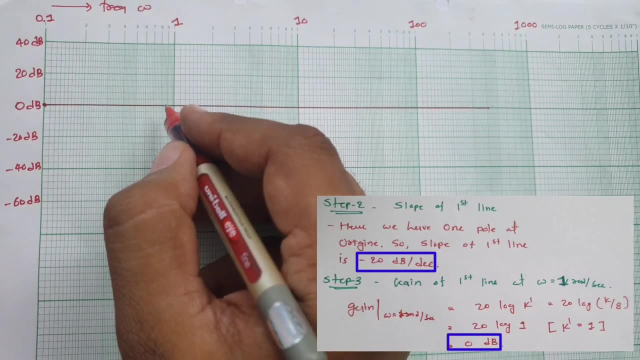 So, as per the calculation, if you see, our first line is having slope minus 20 dB per decade And gain is 0 dB At. omega is equals to 1 radian per second. So omega is equals to 1 radian per second. that is this. 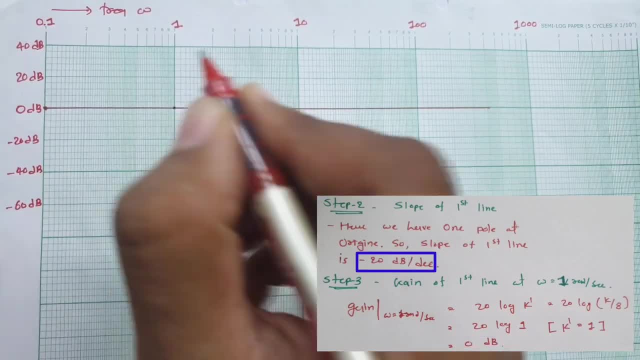 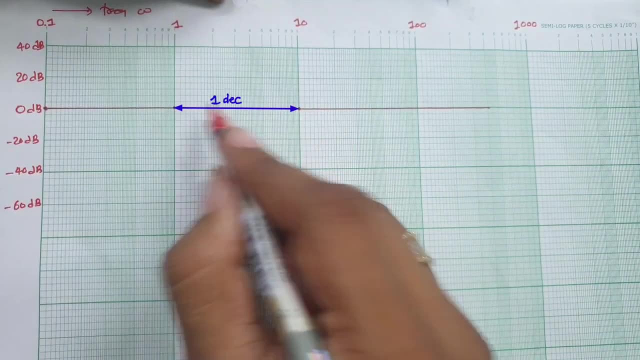 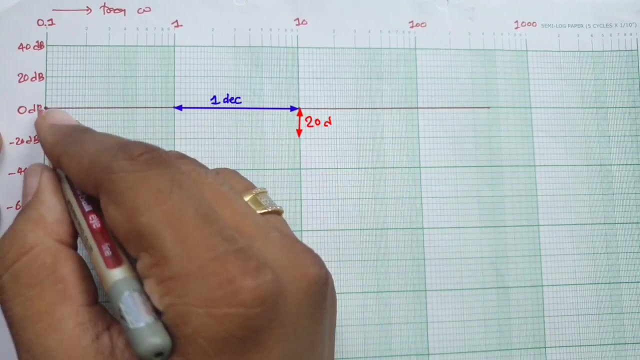 So that point is over here and slope is minus 20 dB per decade. So you see 1 to 1 over here. that is happening. So this is 1 decade and you see 20 dB. that is this Right. So if I stretch a line, 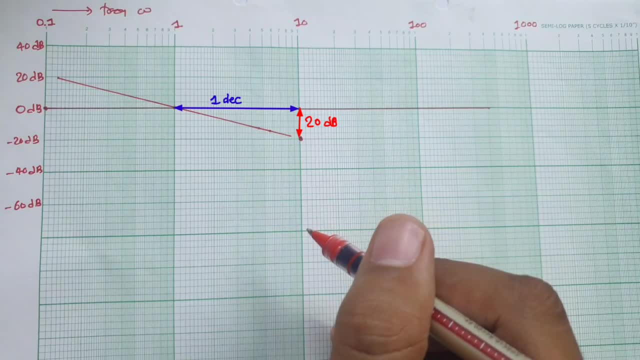 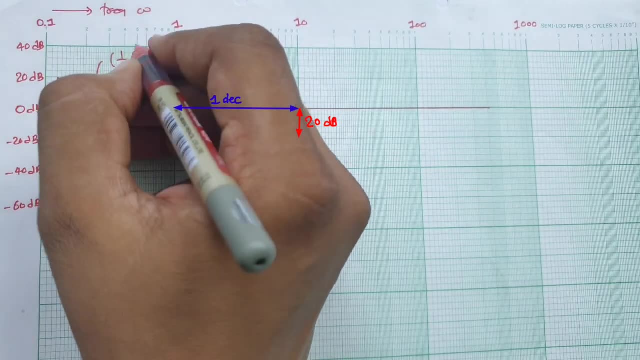 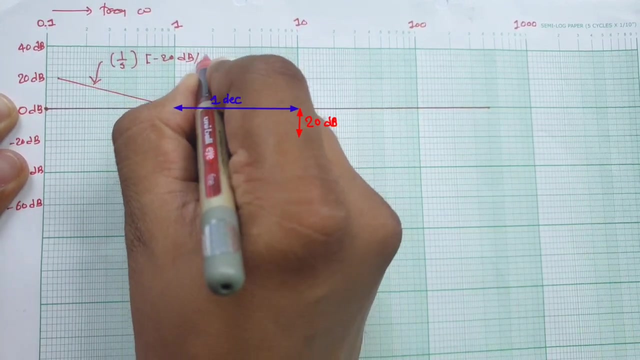 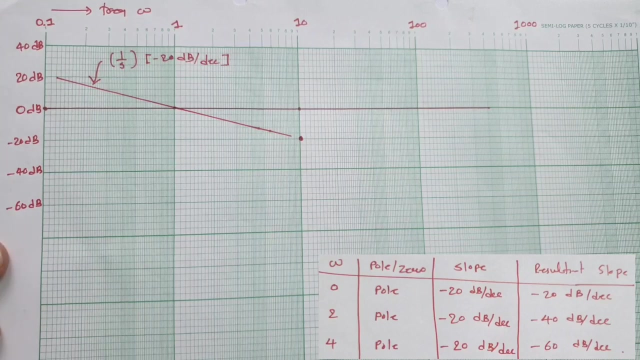 Right, Right, Right. So this is our first line And I can say: this first line is 1 by S. Right, This first line, that is 1 by S and that is having slope minus 20 dB per decade. Now, if you see the table in that second corner, frequency, that is, omega, is equals to 2.. 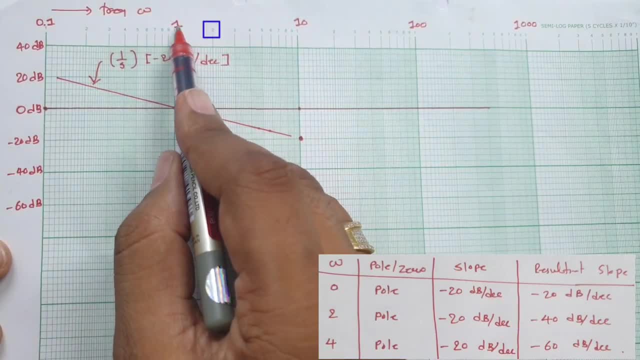 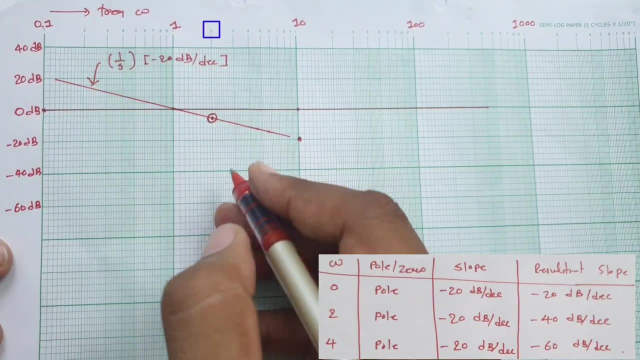 Right, So omega is equals to 2. that is happening, You see. this is 1 and this is 2.. So omega is equals to 2. that is happening over here. So make a point. And that is having a slope minus 40 dB per decade. 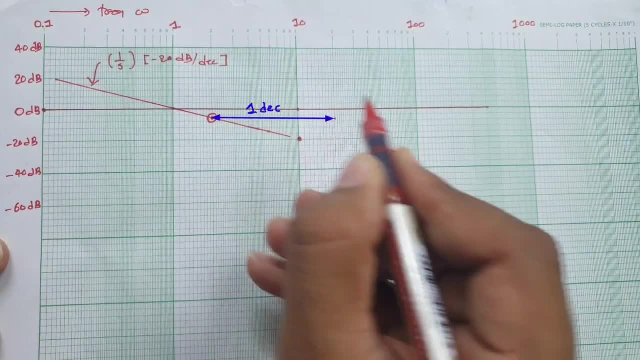 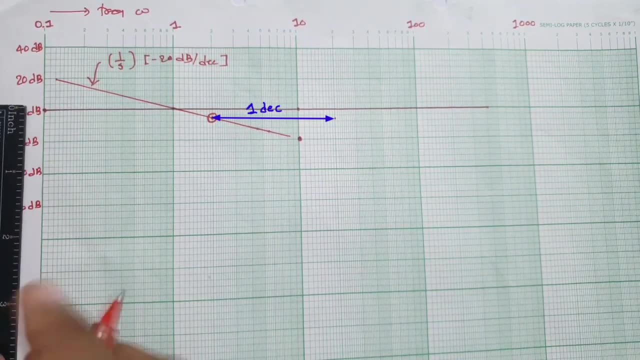 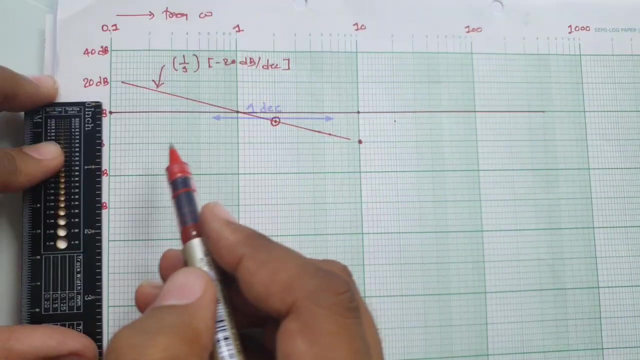 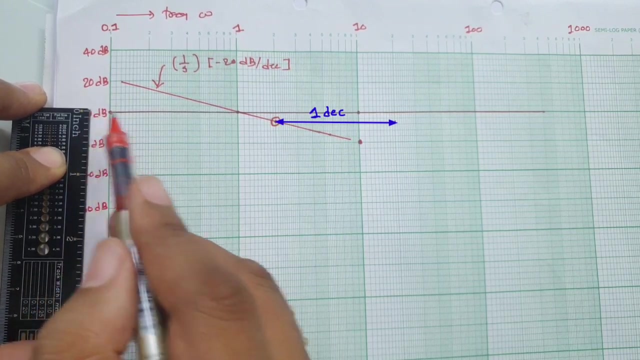 Right. So 2 to 2. that is happening over here And here. all you need to do is you just need to see a scale. You see here, Here to here, there is 1 inch. Right Here to here there is 1 inch, and 1 inch is equals to 40 dB. 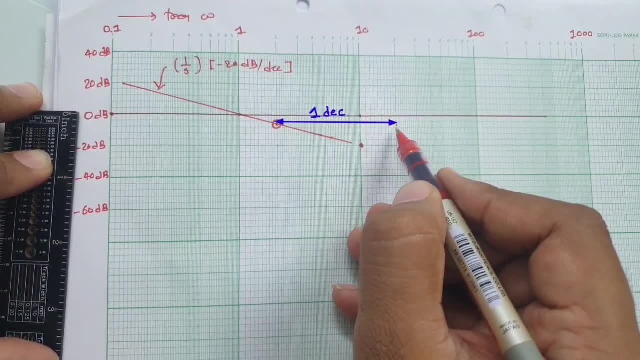 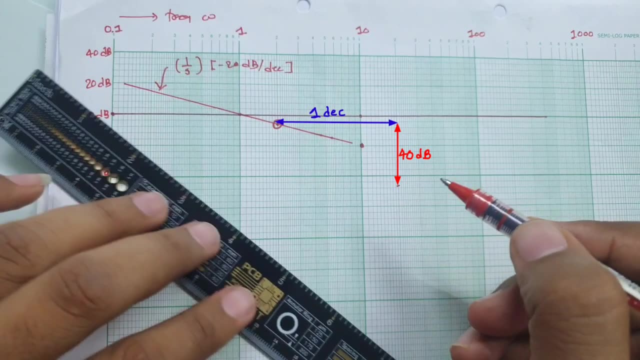 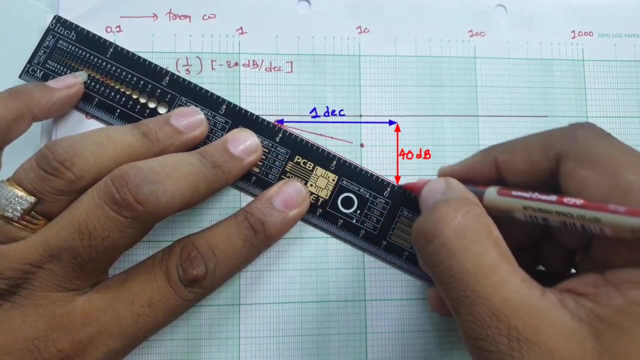 You see Right. So here, 1 to 1, that is, there is 1 decade, and 1 decade to 1 inch, there is 40 dB, And if I have a line from this, Then this line is having a slope Which is minus 40 dB per decade. 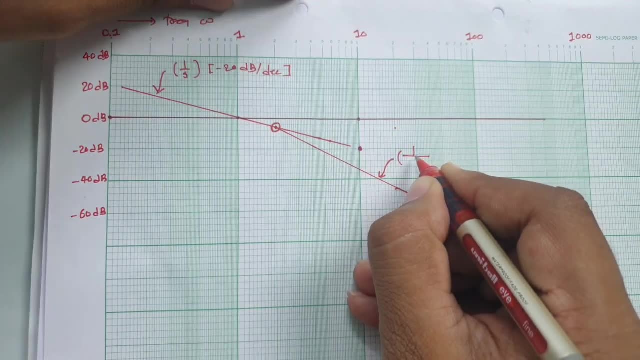 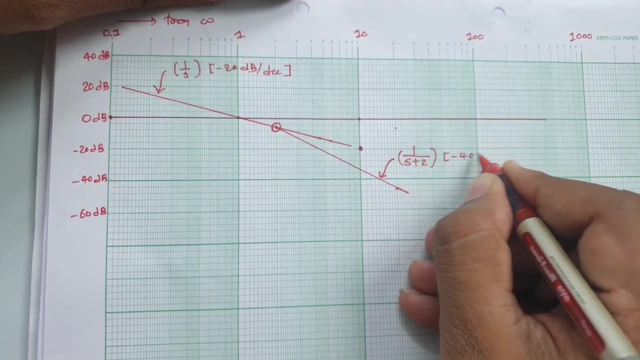 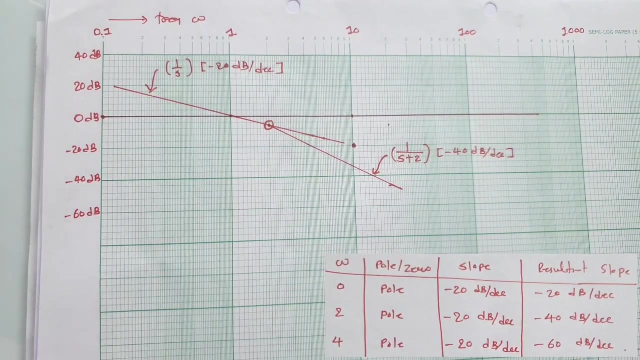 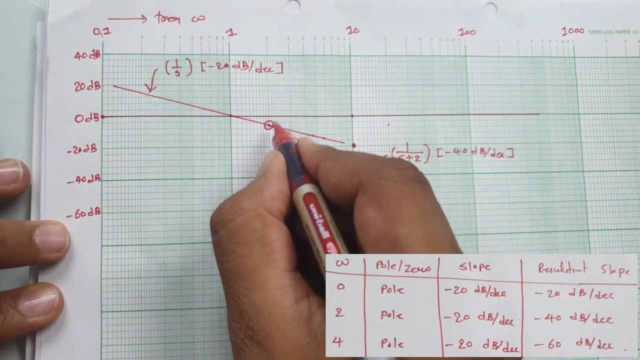 And this is our 1 divided by s plus 2 line, and that is having slope minus 40 dB per decade. Now, if you see our next corner frequency, then that is happening at omega is equals to 4.. So you see, This is 2.. 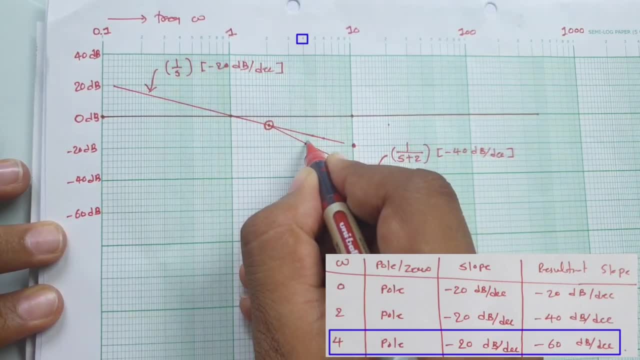 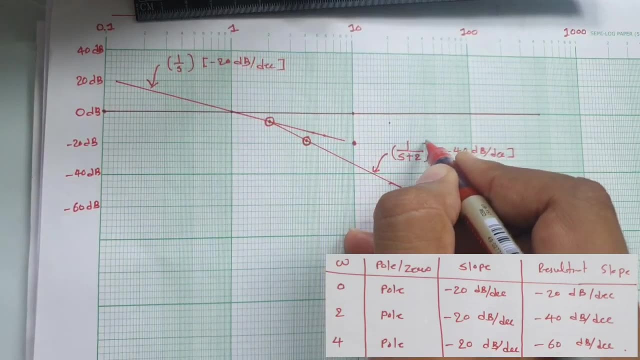 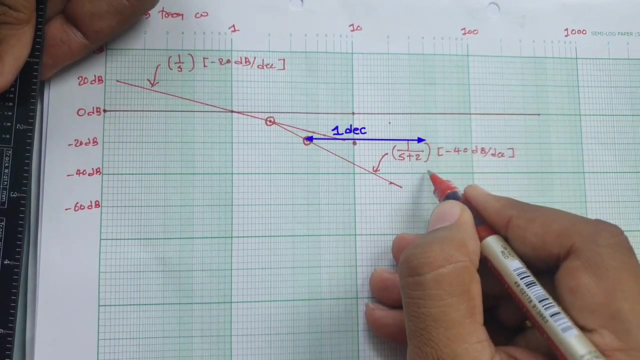 This is 4.. Right, So that is happening somewhere over here. So make a bubble Now: 4 to 4, somewhere over here, and 60 dB, So that I need to say So: here to here, 20, here to here, 40, here to here, 60.. 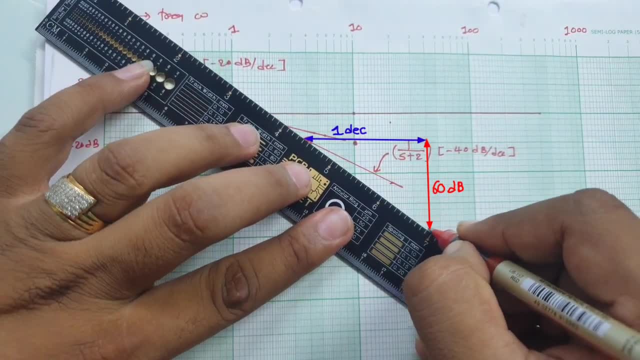 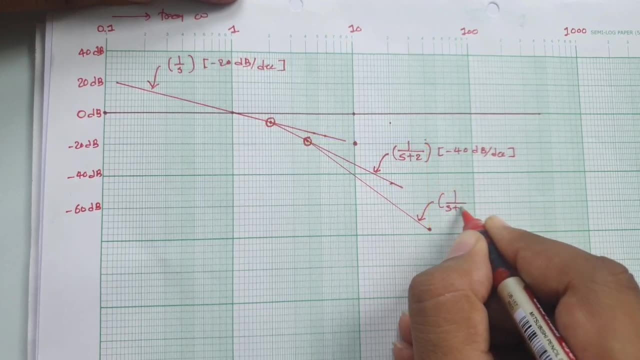 Right, So all I need to do is I need to stretch a line from this, And this is our third line, Right? So that is 1 divided by s plus 4 line. That is 1 divided by s plus 4 line. 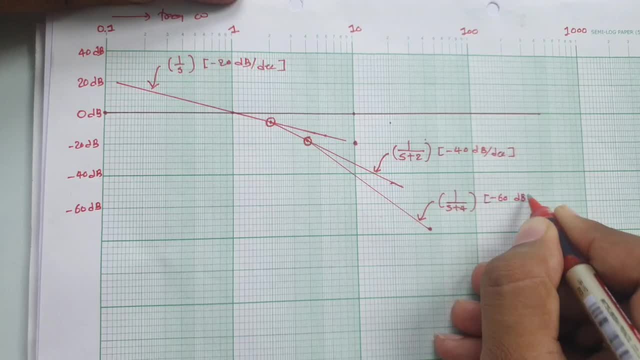 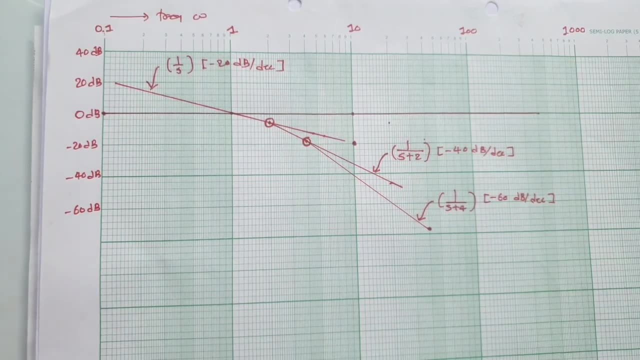 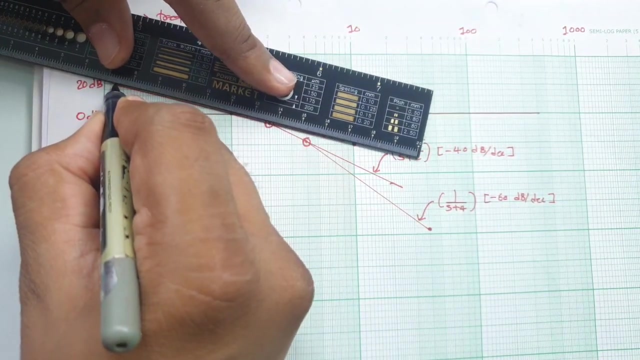 That is having a slope minus 60 dB per decade. So this is how we can have a gain, plotting Right, And in this Let me tell you See Actual gain plot: That is corner frequency to the corner frequency only. So that is this. 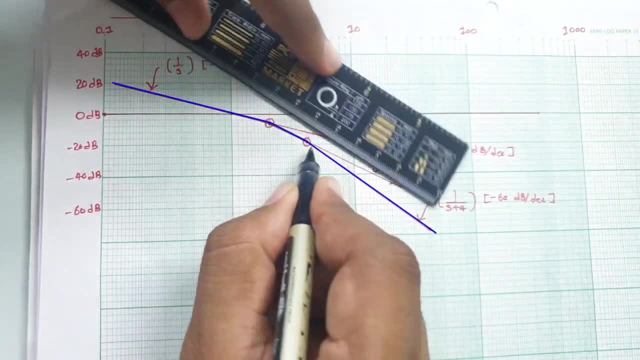 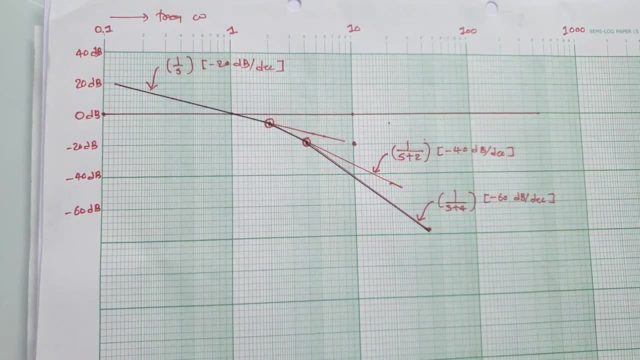 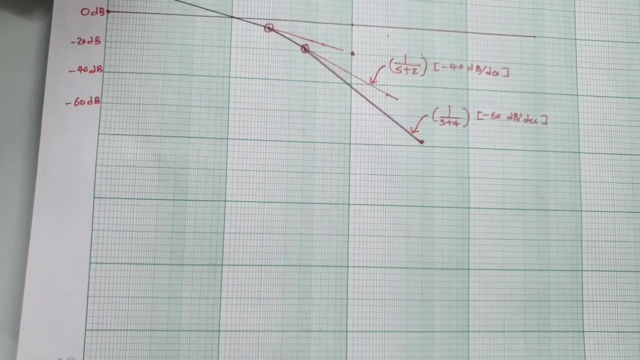 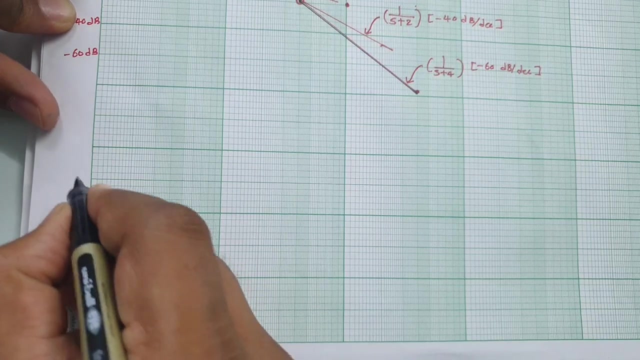 These are just extension, Right, You see. So this is our actual gain: plot plot that one should know right now, let us have a phase plotting. so for phase plotting, all I'll be doing is I'll be considering minus 180 degree over here here, minus 150, here, minus. 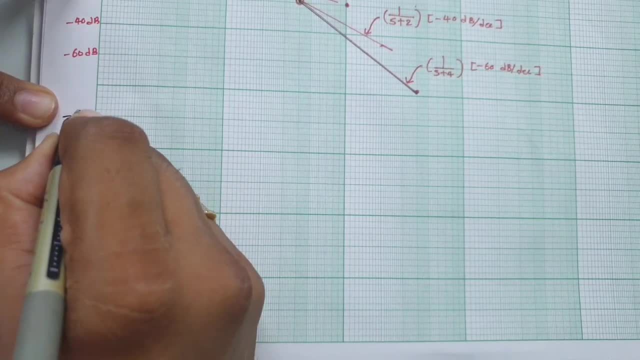 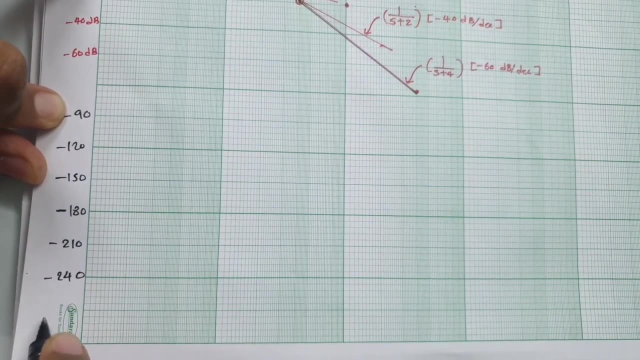 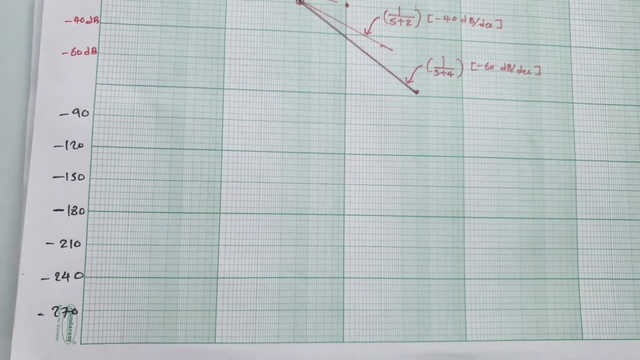 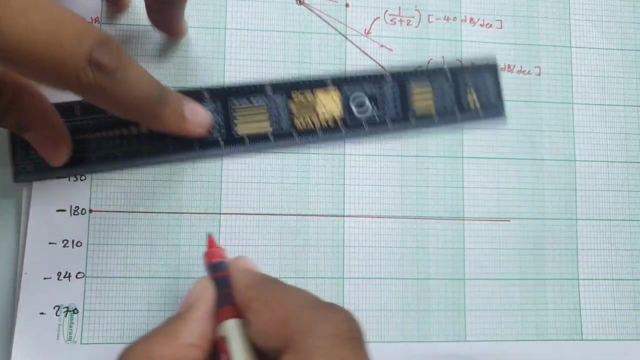 120. here there is minus 90. here there is minus 210, minus 240 and minus 270. this is how it is there, and see minus 180 degree. that should be our reference. so for phase crossover frequency, I need to have this. I am stretching a line from minus 180 degree right now, if you see the table. 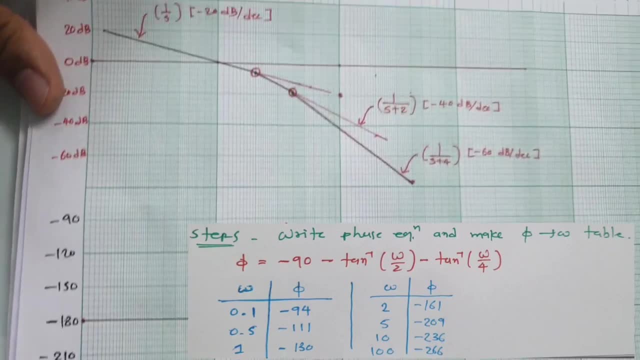 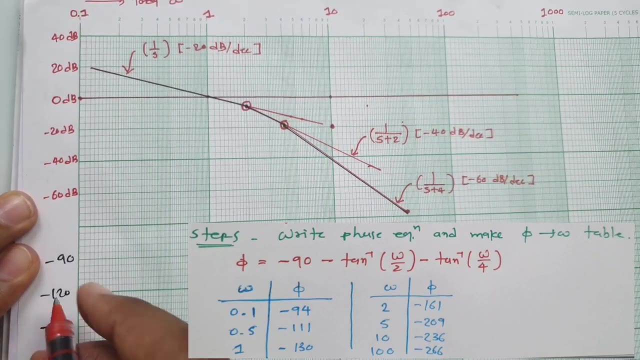 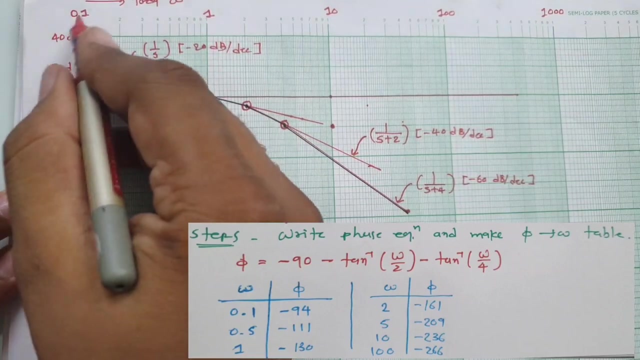 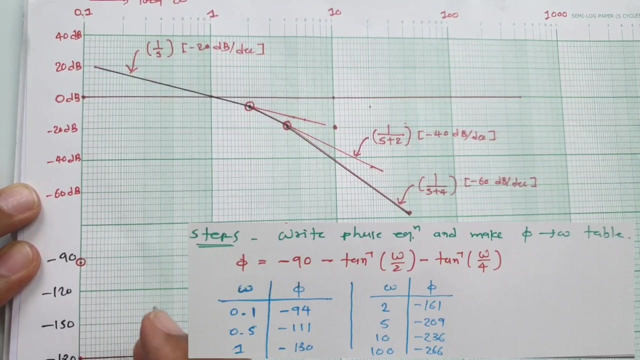 which we have calculated. so as per the table, we need to place values. so at 0.1 radian per second point is some point is there at 94, so that is somewhere over here. 0.1. that is this. you see. then at 0.5 angle is triple one. so at 0.5 means 0.2, 0.3, 0.5 over here. 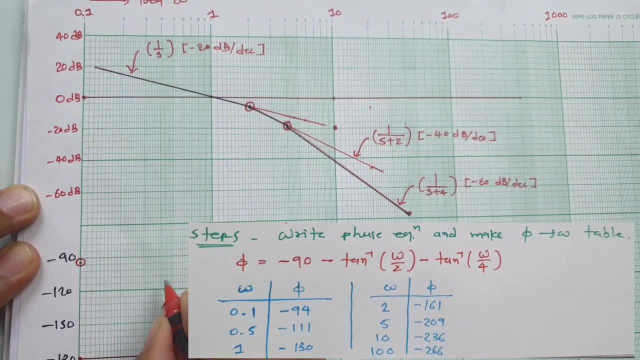 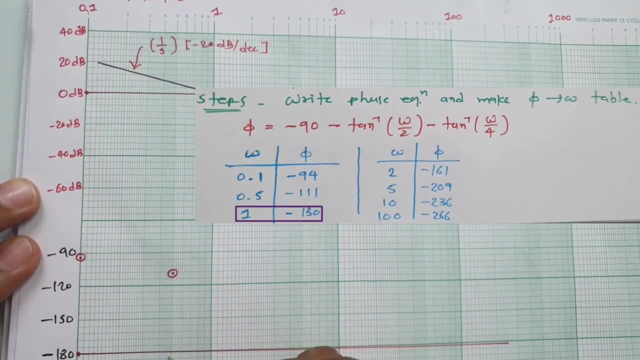 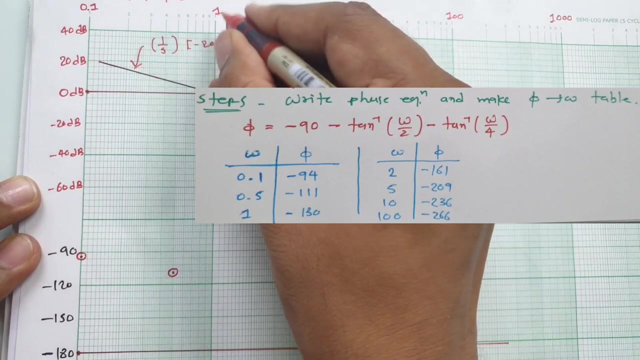 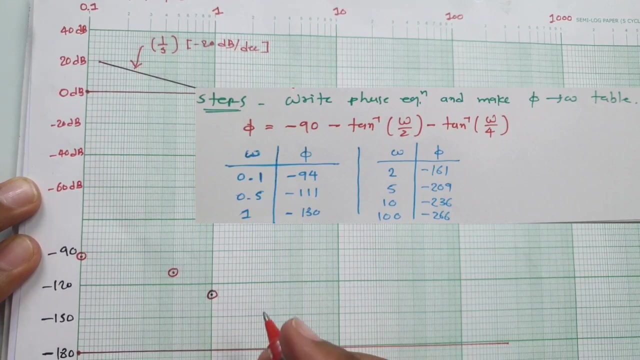 triple one. that is somewhere over here. then next point that we have seen, that was at one and phase was minus 130. so minus 130, see, this is one frequency, and minus 130, that is somewhere over here. and then at 2 it is 161. so at 2 it is 161. 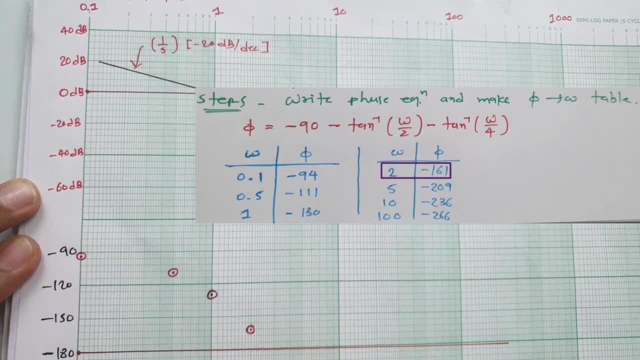 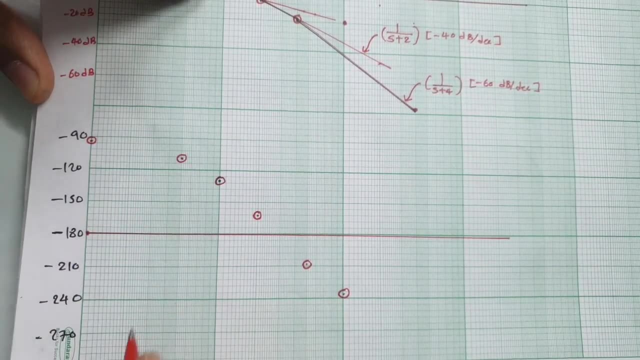 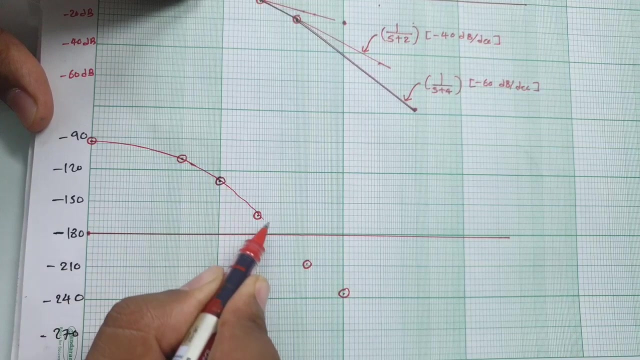 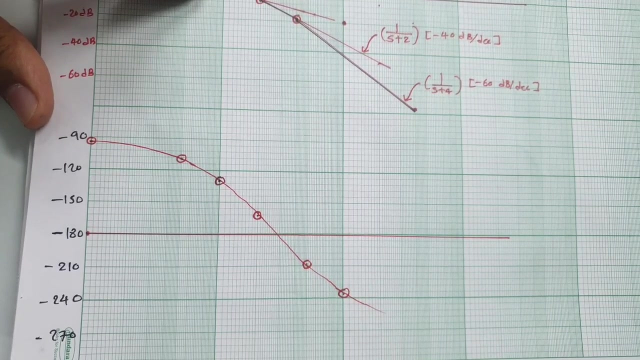 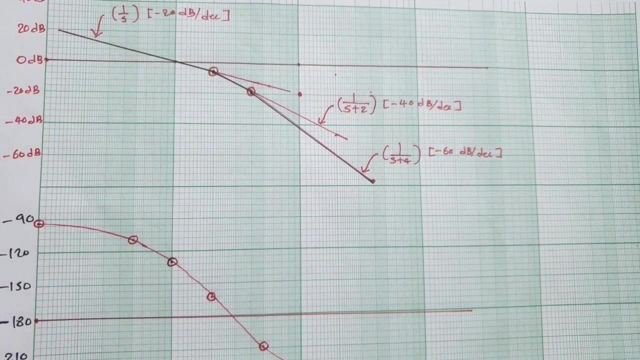 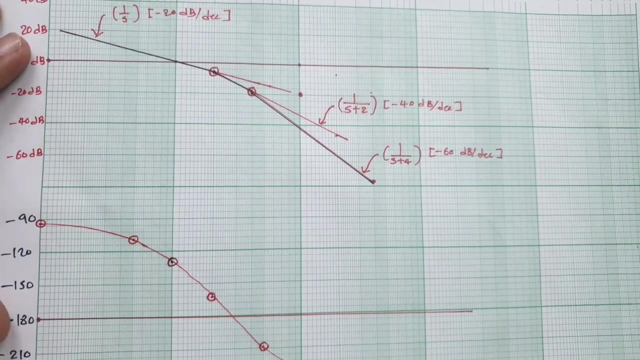 somewhere over here. now from this points, all I can do is I can just stretch a line from this. if you want higher precision, then you can take more points right to have higher precision. now we have this graph: is what body plot graph now from this graph right now: see if you consider K. 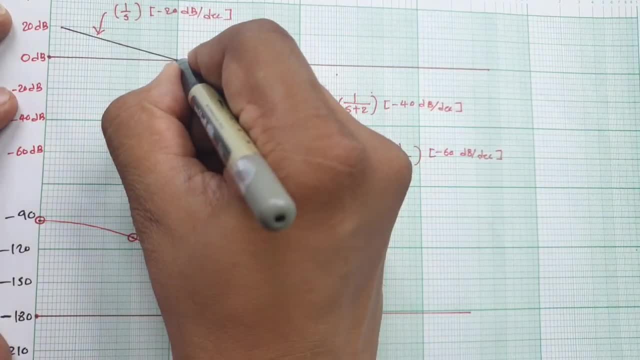 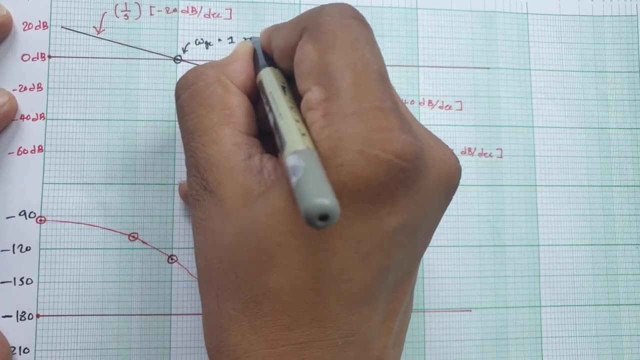 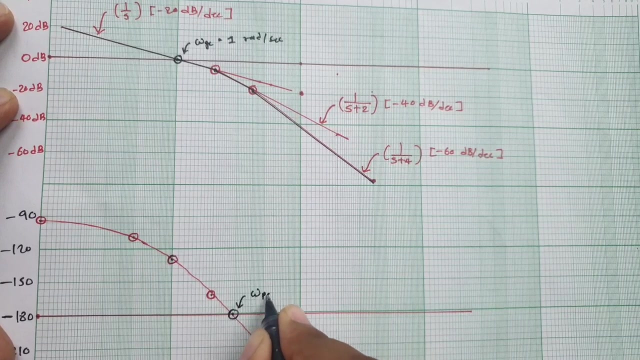 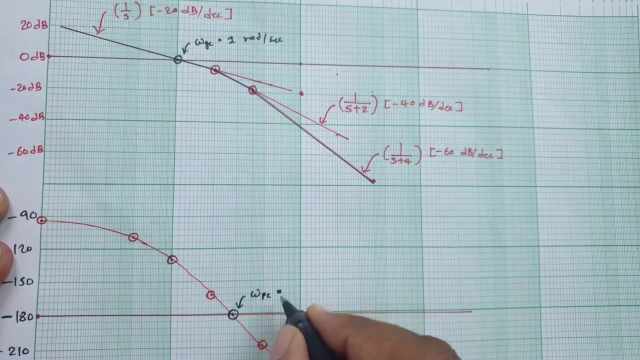 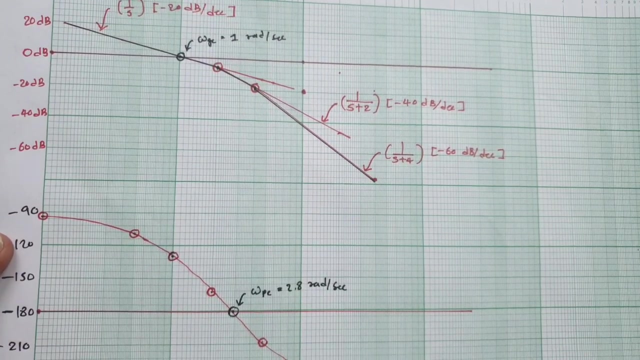 dash is equals to 1, then this is what our gain: crossover frequency, that is 1 radian per second and this is our phase cross, our frequency that is. you see, that is very nearer to 3, but little lower than that. so 2.8, right, and if you stretch a vertical line, 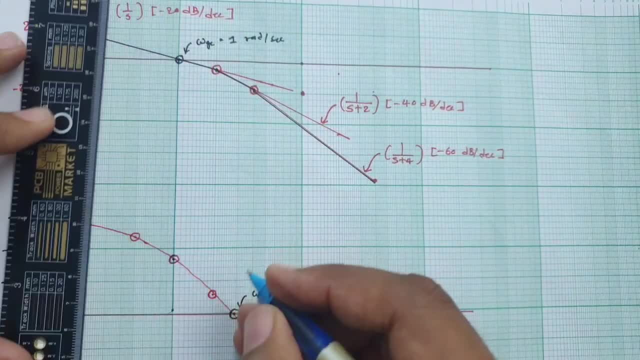 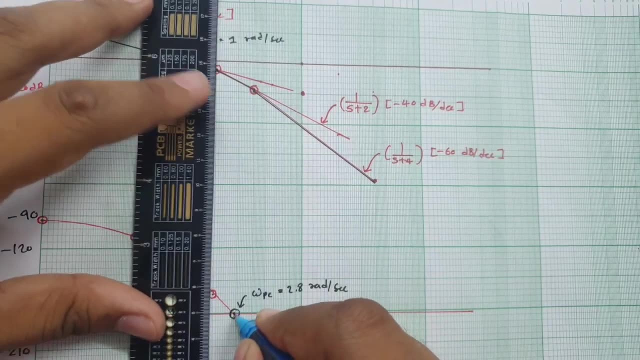 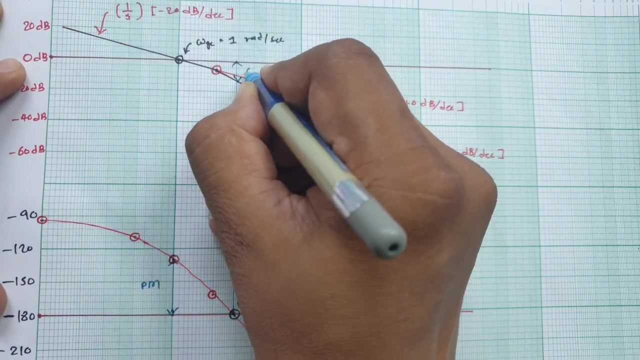 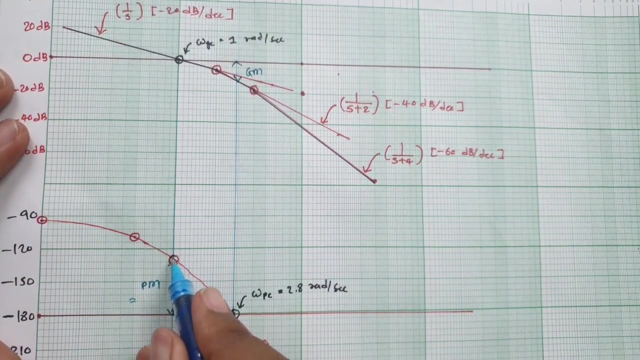 like this right, then this will be our phase margin. and if you stretch vertical line from this, this will be our gain margin. and if you see phase margin, then that is you see 30 plus 20 approximately, so I can say that is 50 degree. and if you see gain margin, 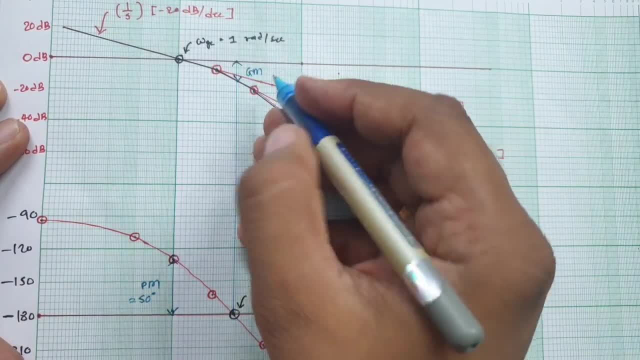 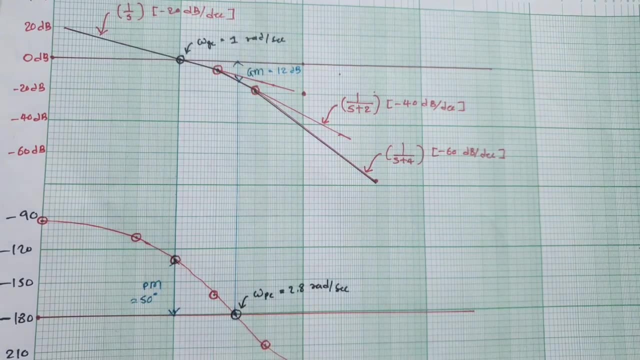 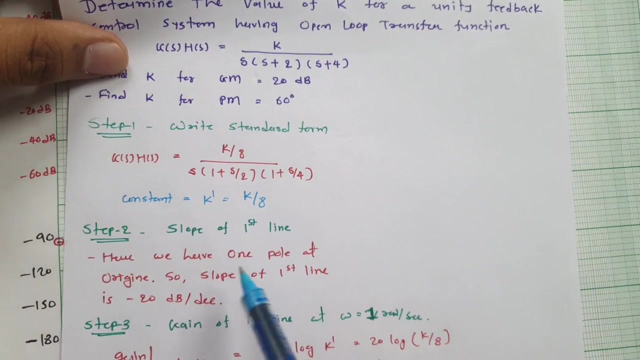 So for five boxes it is 20, so for three box it is 12. so I'm saying gain margin is 12 dB and this is what we have. for which values? this is what we have, for K dash is equals to 1, right, and if you see K dash, that is K by 8, right, and that is what we have kept. K dash is equals. 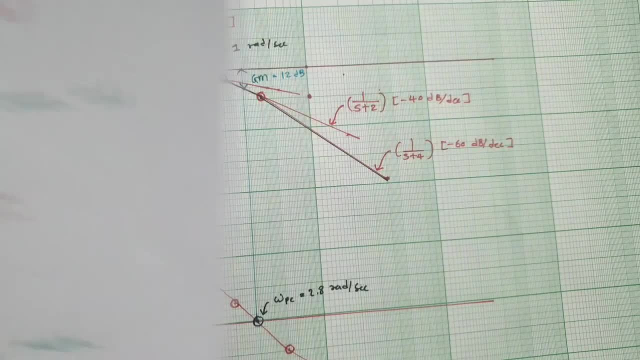 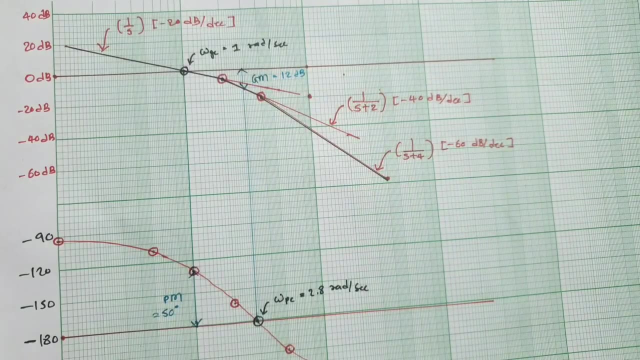 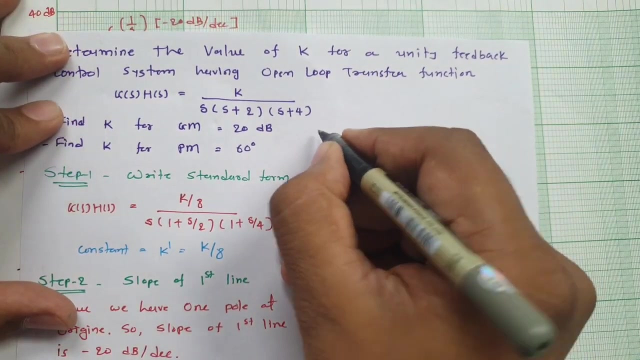 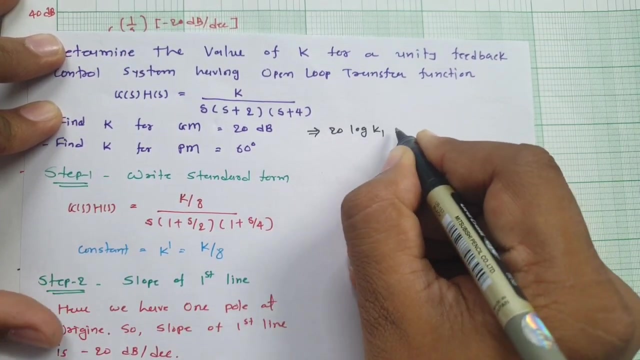 to 1 to have this plot Right Now, our question is: find K for gain margin is equals to 20 dB, right? find that gain margin, find the value of K for gain margin is equals to 20 dB. So how to calculate this? so you see, to calculate that all we need to do is 20 log of K, 1 that 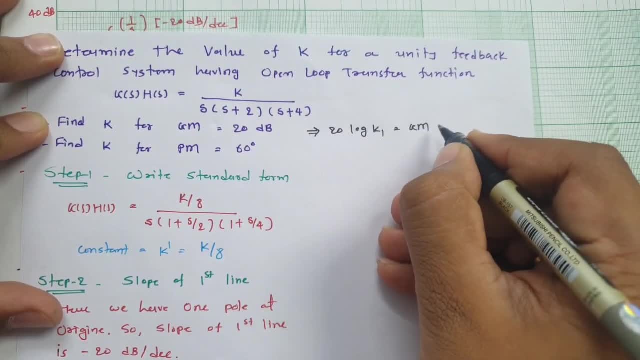 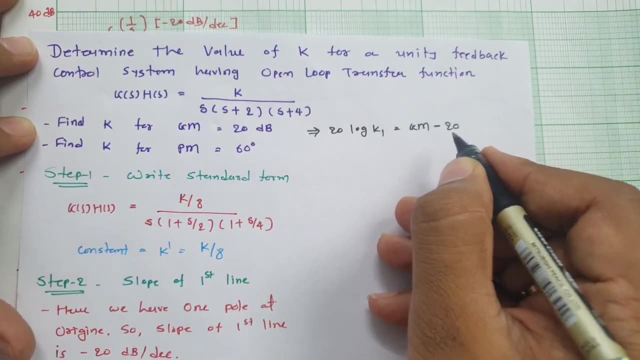 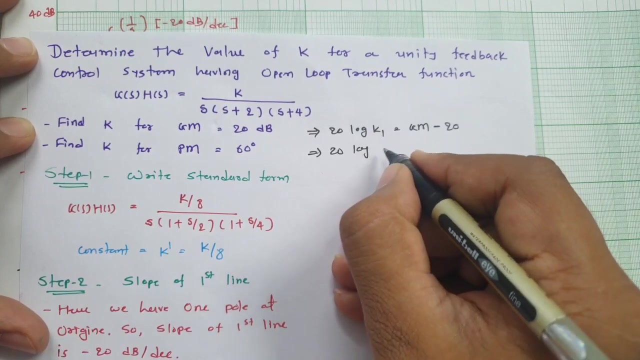 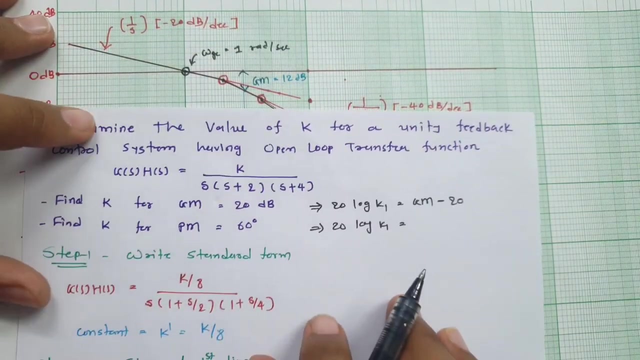 should be equals to Gain margin minus 20, see 20 that is required. so actual gain margin minus 20 that we need to do, and here 20 log of K 1. you see gain margin over here we have calculated that is 12. so I'm saying this is 12 minus 20.. 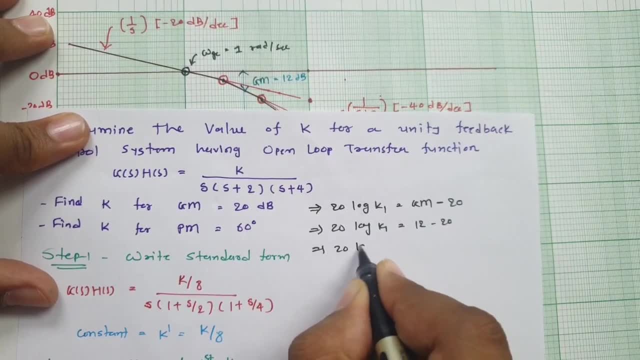 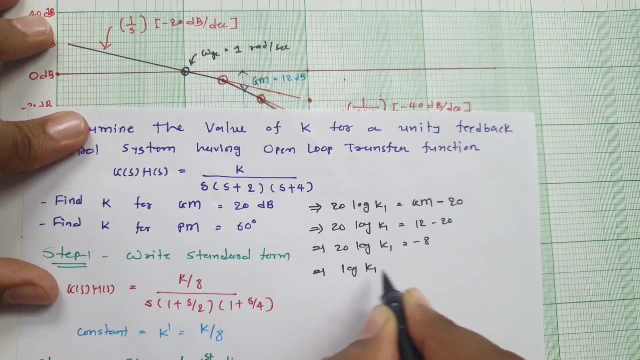 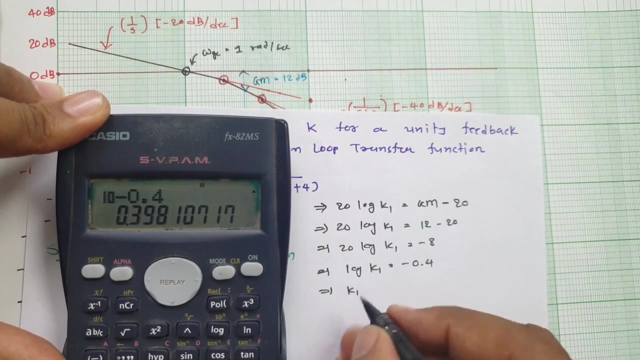 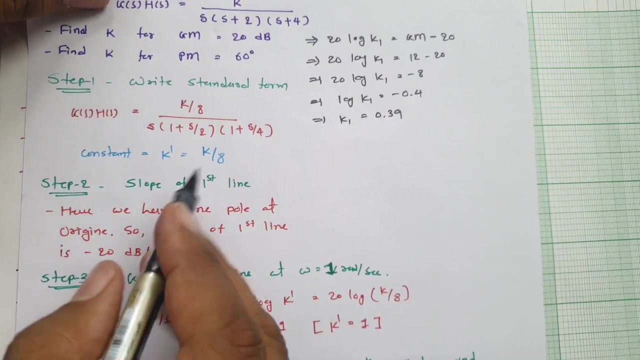 So I can say: see 20 log of K 1 that is minus 8. so log of K 1 that is minus 0.4. so we can have K 1 and K 1 is 0.39 and if you see K 1 is K, 1 is K by 8. sorry, I have written K. 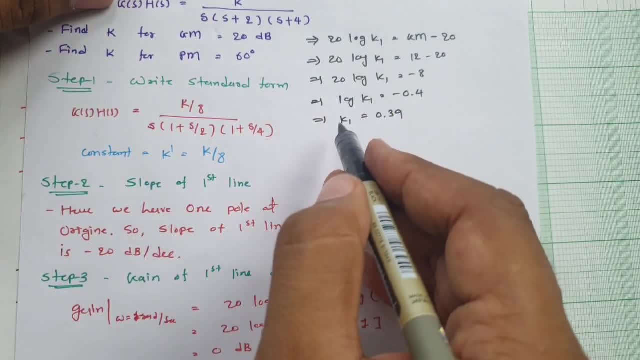 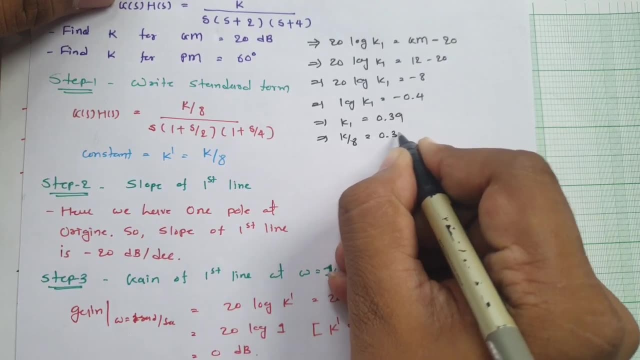 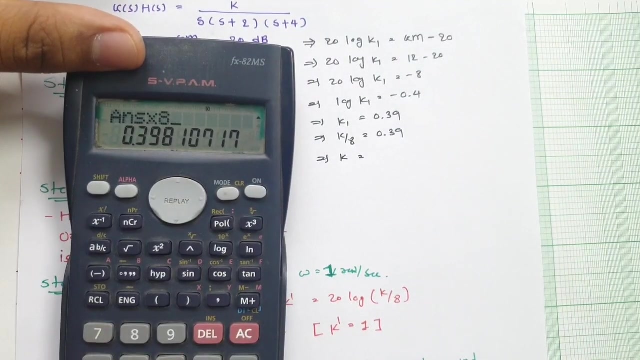 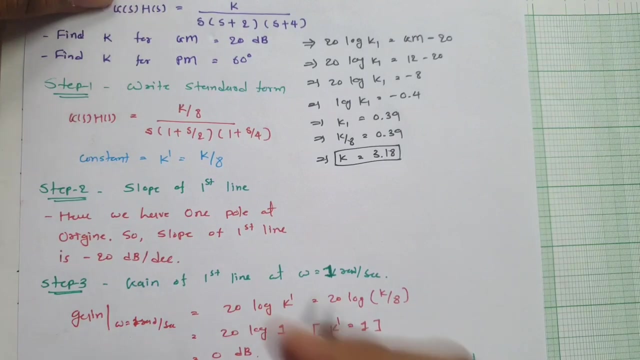 1. That should be K dash. so K dash is K by 8. so multiply by 8 that we need to do to have value of K, so 3.18. this is our first answer for K 3.18, if gain margin is 20 dB now second: 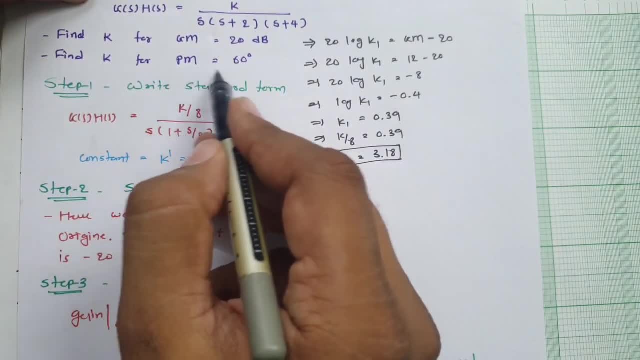 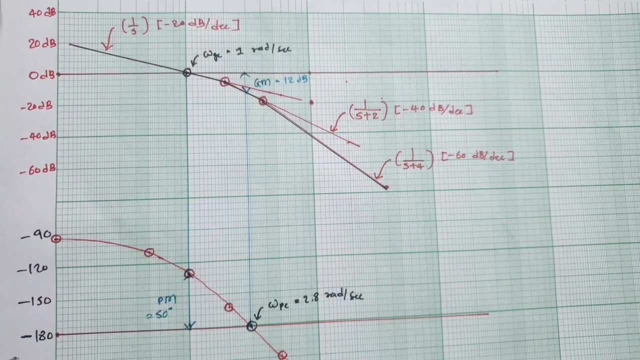 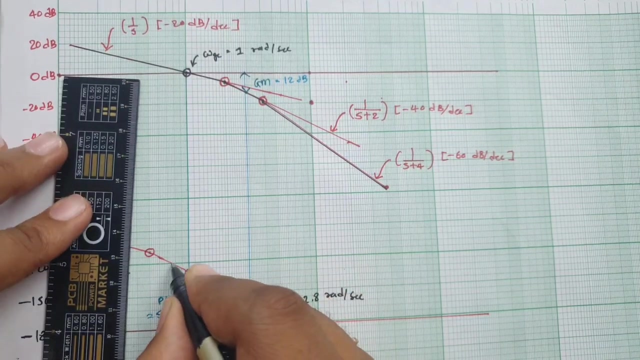 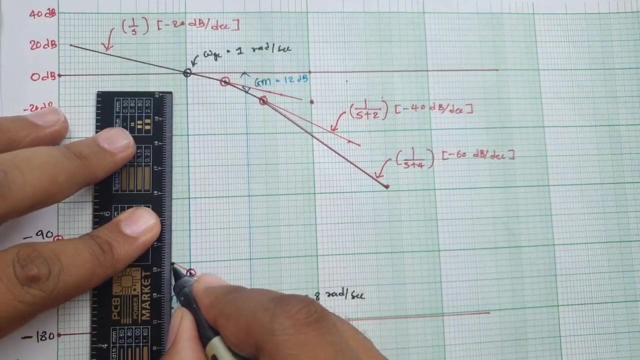 question, that is what find a k for face margin? that is 60 degree, right. so first of all, we need to see at what location it is 60 degree, right? so i'm just observing it is happening somewhere over here, right? 60 degree. you see 180 to 120. so this is what: 60 degree face margin. 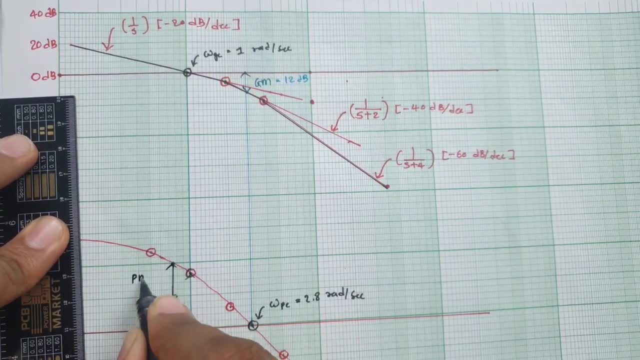 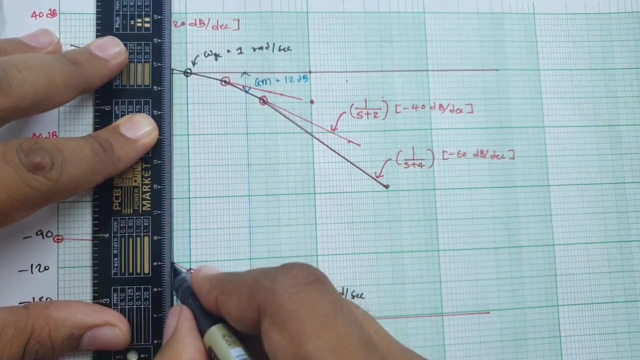 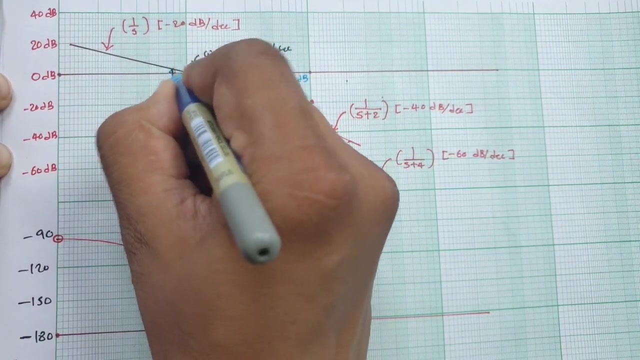 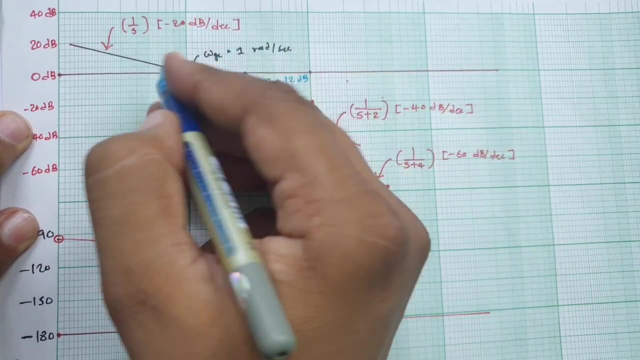 right face margin is equals to 60 degree if you stretch upward line, and that is happening like this. so here all we need to do is we need to see how much value is there with this right. so that is approximately. one can say it is 4 right gain margin. that is approximately 4. now here there are 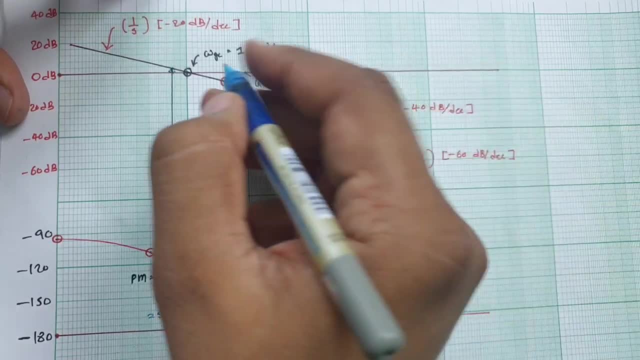 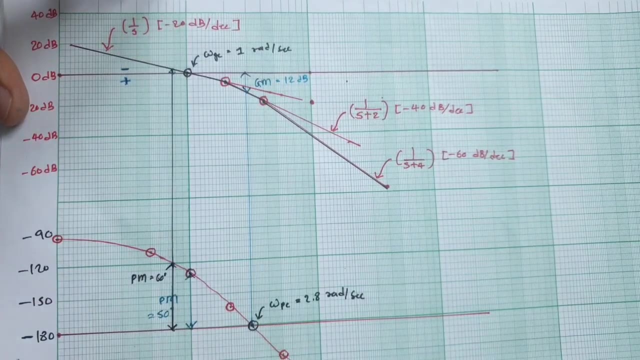 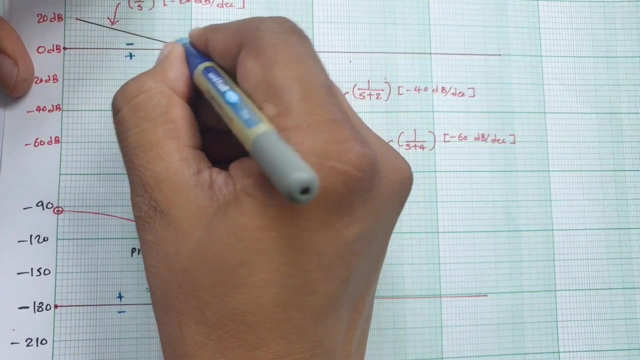 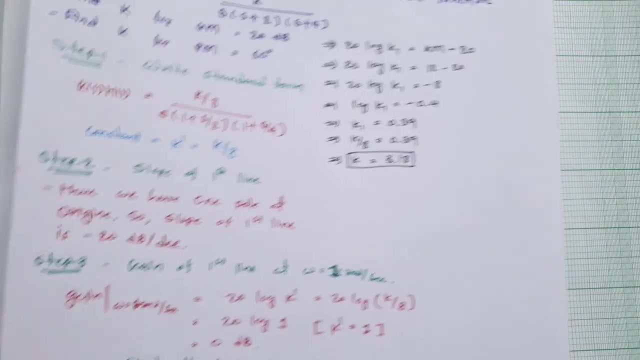 few points that one should know: see gain margin that is negative over here and positive over here, and face margin that is positive over here and negative over here. right so this is our gain margin. that is minus 4 that one can say over here, right? so what i'll be doing is for a calculation of k. i'm considering